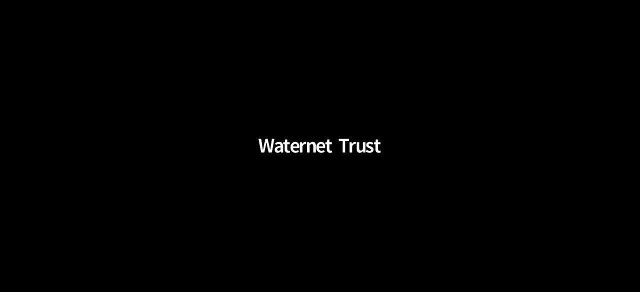 Or if you have any comments on how we are running the course, please proceed. You can provide us with feedback in the chat box, So we'll start the meeting at five past, as we give more people an opportunity. Then those who were asking about how to submit assignments like the assignment given yesterday: 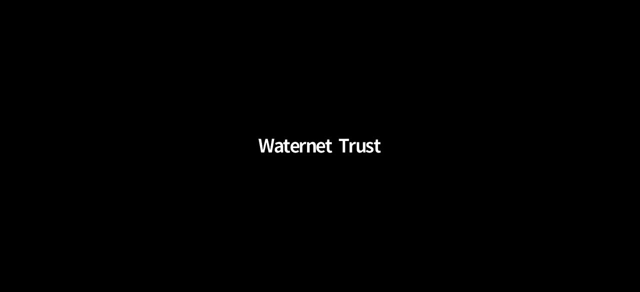 we will send you an email, But we now have a feature on the platform where you can submit the assignments. We will let you know and send you the submission link, And the lectures are being recorded. We have uploaded the one for yesterday on YouTube. 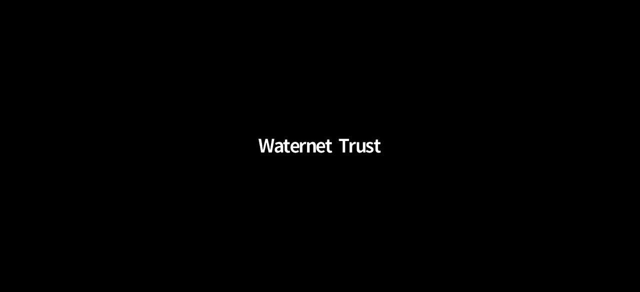 So you should be receiving it. We are receiving a link for yesterday's lecture, and this one will also be uploaded on YouTube. Thank you, If anyone has a comment, as we wait for the other people to join, please feel free. Let's be interactive. 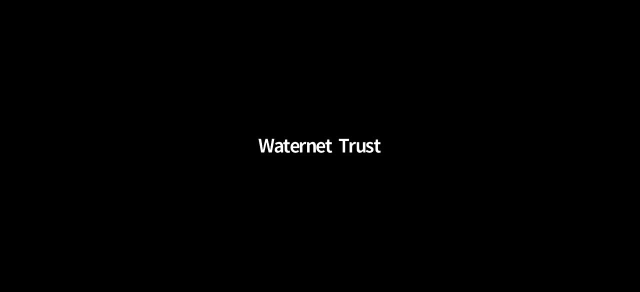 Just interject and say out your comment or question, Or maybe you just want to introduce yourself. Please feel free to do that. We have one minute before we start. Can you hear me? Yes, we can hear you. Okay, Yesterday I think you were given two assignments. 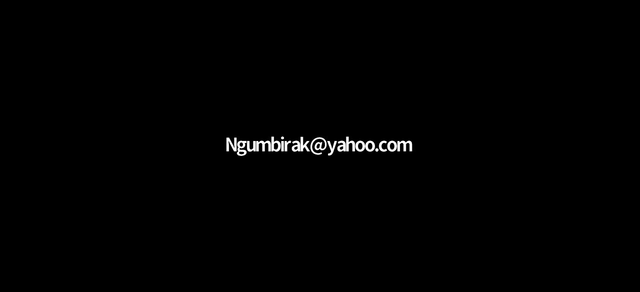 I'm not sure if you said that one was submitted today and the other one was submitted tomorrow. Is that what you said? I'm not the one who was delivering the lecture yesterday. I can ask Mr Gumindoga, but the issue was about the submission. 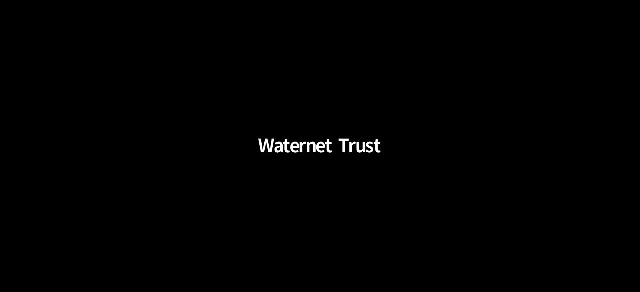 But now the submission portal is there, We'll circulate an email with the dates on when you can submit the assignments. Okay, Yes, One thing that I want to clarify. Okay, come again. I want to do one thing. clarification, one thing. 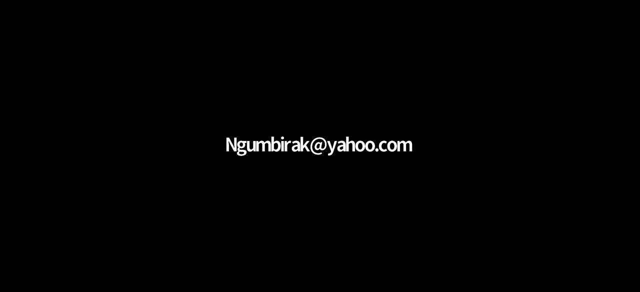 Are we getting a certificate by the end of this course? Yes, you will get certificates. Just write your assignments. Just write your assignments and the certificate will come. Okay, okay, Okay, okay, Thank you. Okay, okay, Okay, okay. 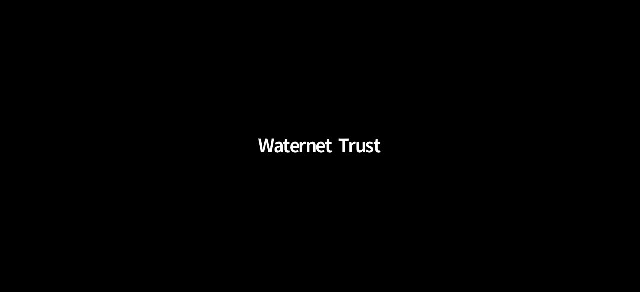 Hello, Hello, Hello, Yes, You can go. Yes, May I ask again? Did you say you will send us the link in where we'll submit the assignments? And again, how do you access Come again. Did you say you will send us the? 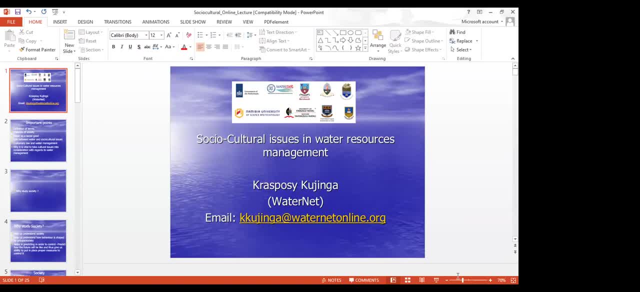 Okay, I'm saying we will send an email on how you can access, on how you can submit the assignments. Okay, And how do we access the yesterday's lecture? We'll send you the link. Okay, Okay, Yes, Okay. 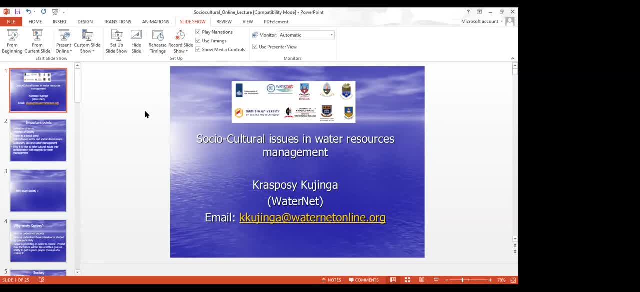 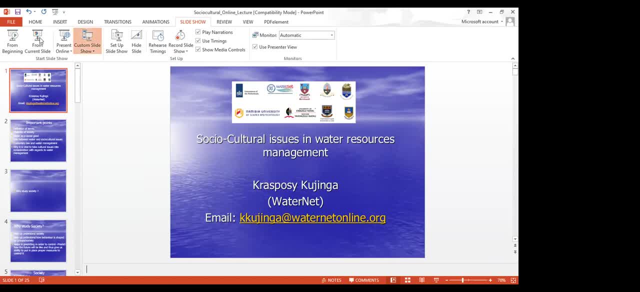 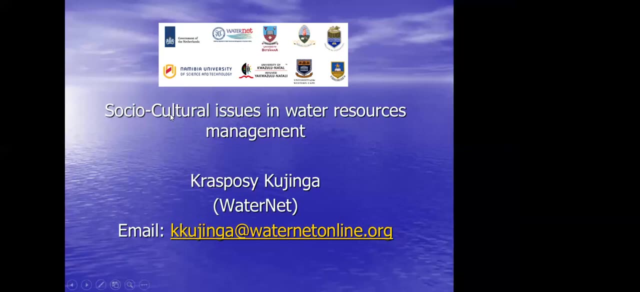 Okay, Okay, Okay, Okay, Okay, Okay, I'm going to put my presentation on slideshow. I don't know what's happening. Okay, I'm sure it's now on slideshow. So today we will look at two areas. 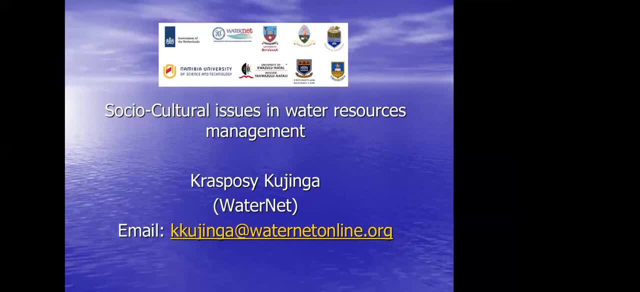 One is on socio-cultural issues in water resources management. Okay, Yesterday you looked at the introductory parts, which included principles of integrated water resources management, So we now want to go further and look at the context within which we do our water resources management, IWRM. 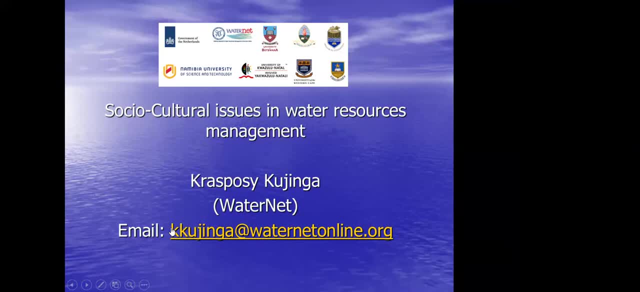 We do this within a certain social and cultural context, Because we are human beings, We are social. We are social beings, We live in societies, a society with a society with their own culture. Could we please mute our mics and Moria? kindly ensure that everyone is muted. 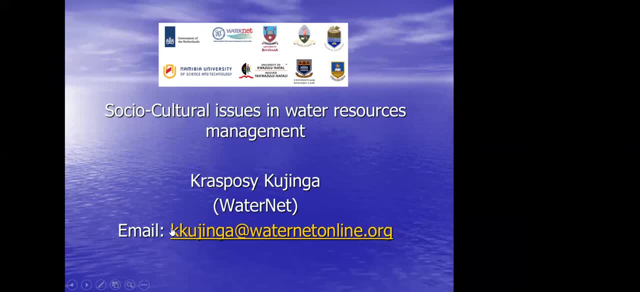 So we just want to look at the basic concepts Of what is society, What is culture, And also, briefly, on the theories which inform society and culture, And once we do that, we'll then have an appreciation. you know that it's always important when 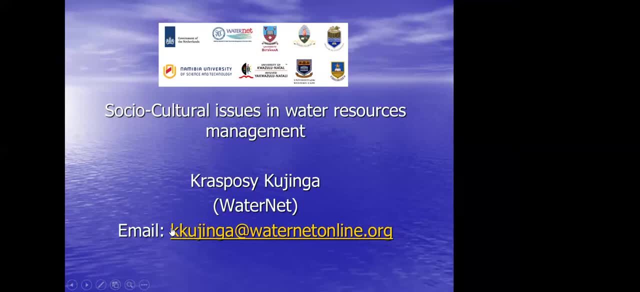 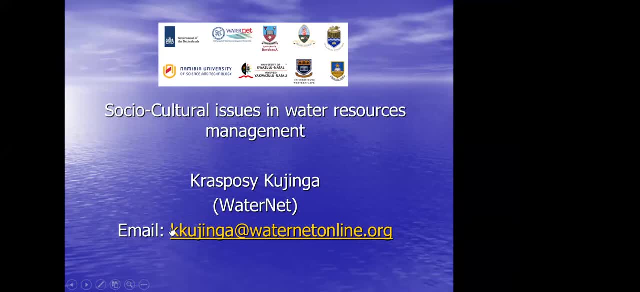 that we are operating in. Maybe, before I start going down the slides, can anyone help us in defining what society is. What is society? Anyone can unmute. They can unmute if you want. process, Go ahead. Carlson, Wow, Anyone. please can we have an attempt on what society is? 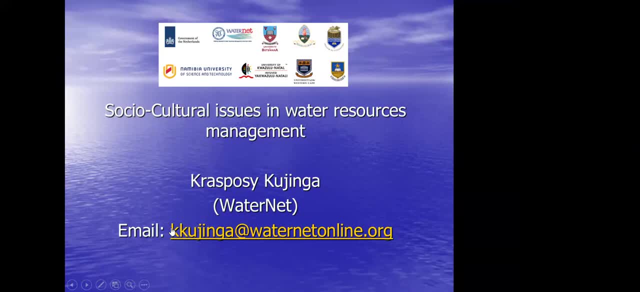 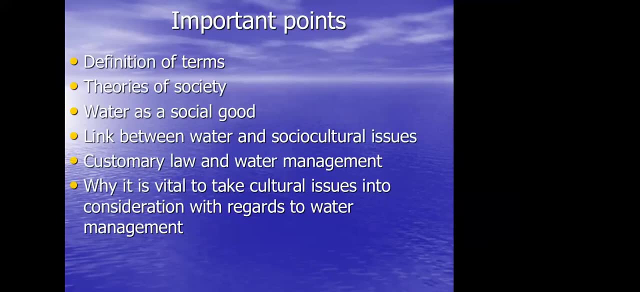 Okay, so that's not just the important points that we need to take into consideration. We are going to define some terms and then we are going to into the theories of society and then a bit about water as a social good. We will not touch on customary law and water management today, but when I circulate the 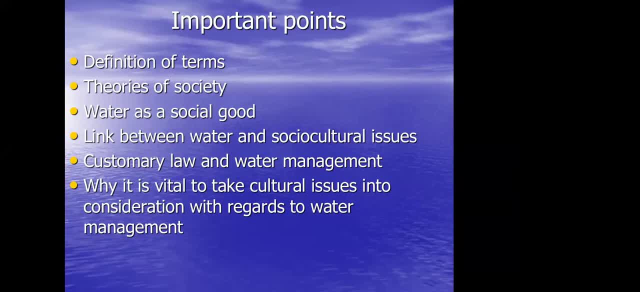 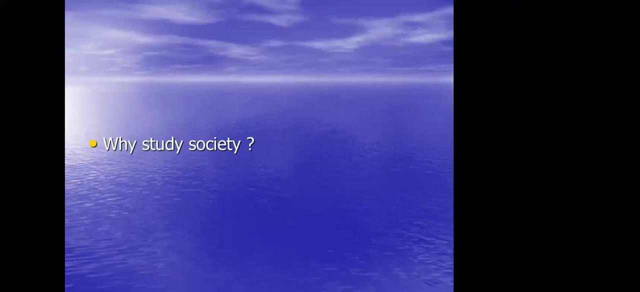 slides. I will circulate with all that information so that you can understand. You can also understand the issue of customary water law. So what we always need to know: when you are an IWRM or a water resources management practitioner, you should always understand society. 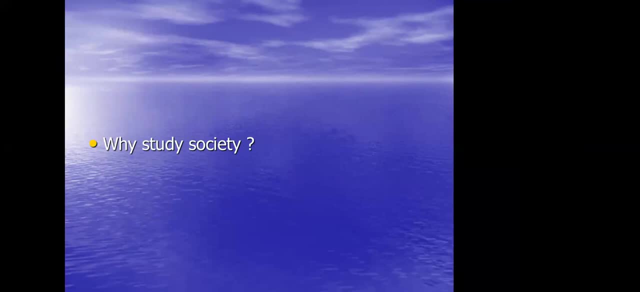 You should always, you know, have a definition. There is no standard definition of society. They are different, As you will see. we have a lot of definitions, but these definitions have something in common, Though they differ in certain aspects, but they have certain, you know, aspects that 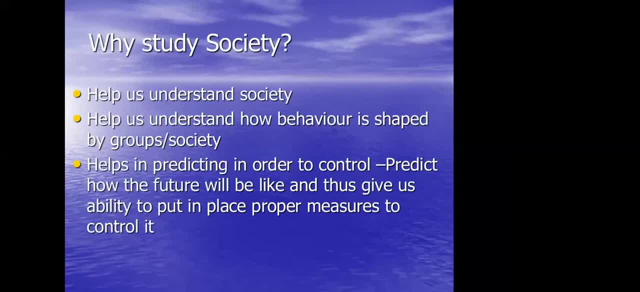 are common. So why should we study society? We live in a society. We want to understand society. We want to understand how that society is shaped and how it is shaped by groups and by the larger society itself. And also we want to understand society has institutions that are in place. 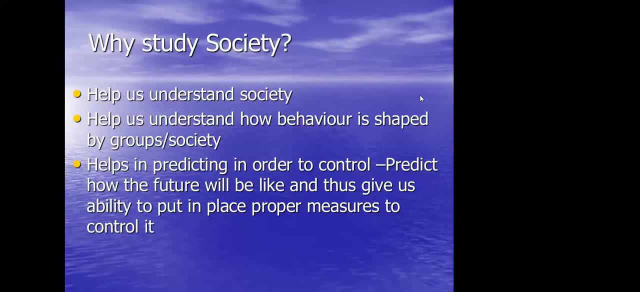 Institutions for water resources management. they are found within society. Society has laws, So we want to understand all those things. How do they operate? How do they work? How do they do? How do they live? How do they do it? 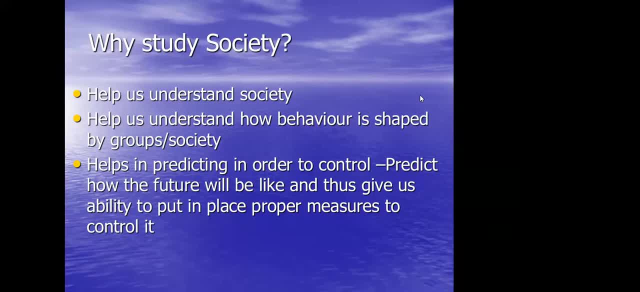 How will they change? What influence their change? You see, because society is not static, society is dynamic, And also it helps us in predicting order to on how the future will be like, And this gives us an ability to put in place proper measures to control it. 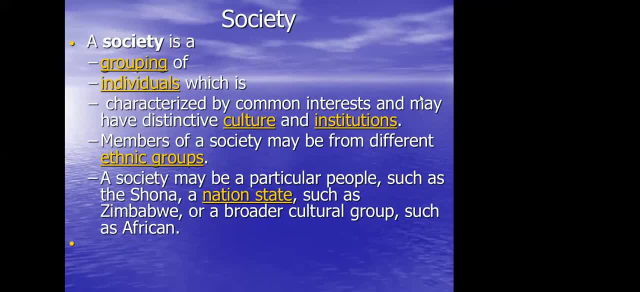 And then, what is society? As I have said, there are different definitions of what society is, So one can define it as characterized by having a sense of what society is, And that is the idea, And that's the most important thing, And that's the way I see it. 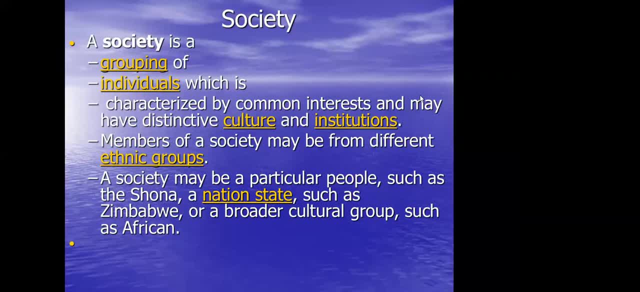 I think that's the best way. I think a lot of people don't know what society is in a sense, But it's not a question of being positive, It's a question of having a sense of what society is, And that's the main thing. 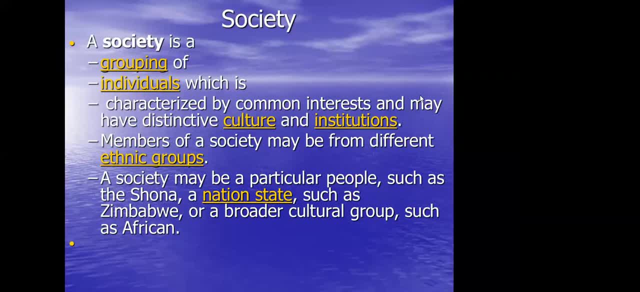 And we're not going to talk about that here. But what society? is the first thing that I would like to say. I don't know if I'm going to go too deep. The first thing I want to say I think there is a question I would like to ask. 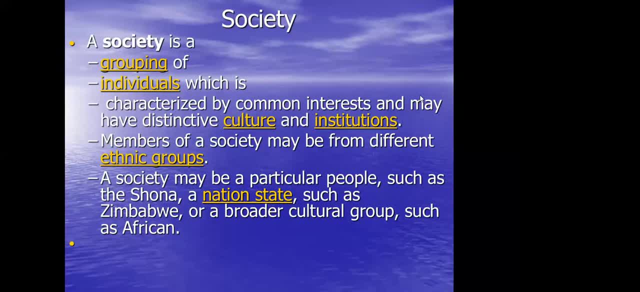 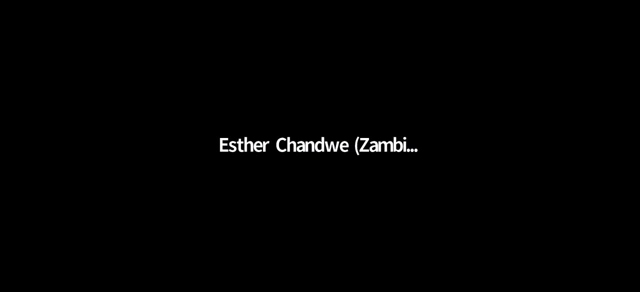 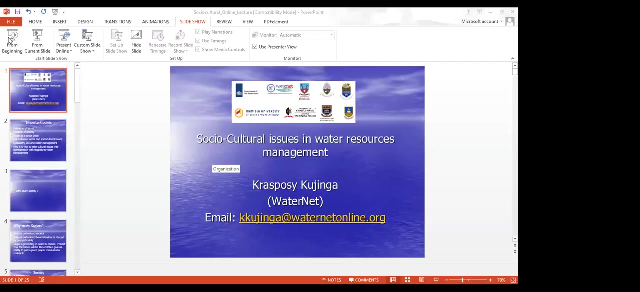 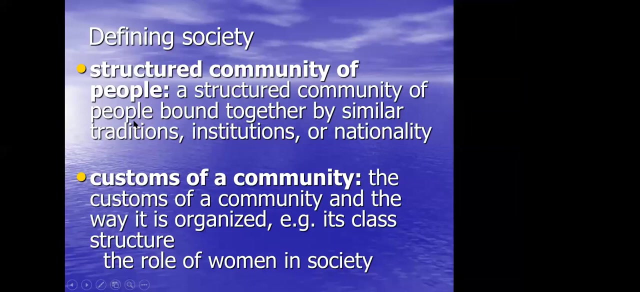 I don't know if I'm going to be going too deep, But I really want to ask you a question: What is society? sorry, i've been- uh, i've been- cut off. so society can be a structured community of people bound together by similar tradition, institutions. 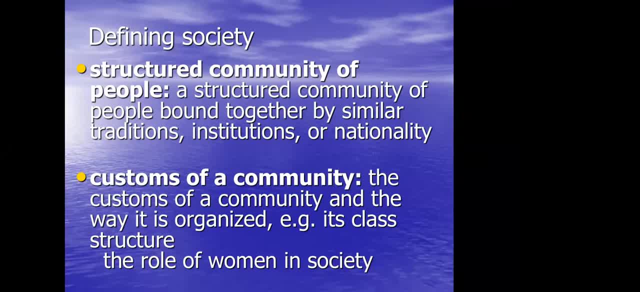 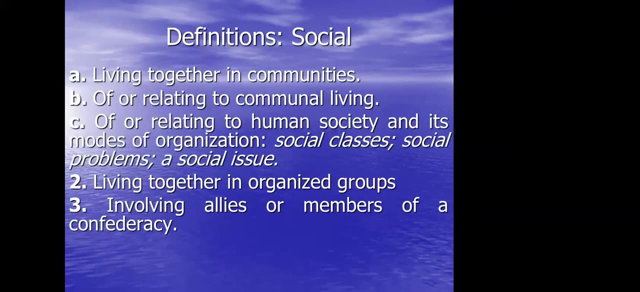 or nationalities, or it can be custom of the people and the way it is organized. it's a class structure and also we need to define what is social, because society comes from the words. it's a french word called socios, which means associating. so society comes from the words. 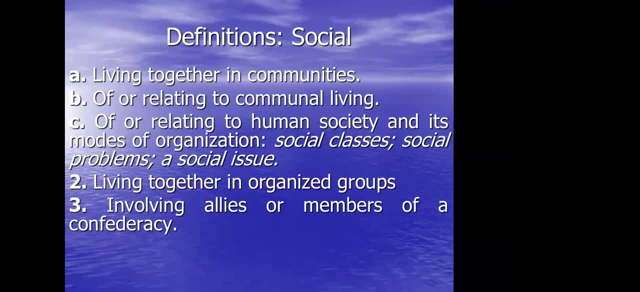 so society comes from the words social. it basically means living together in communities, and when you live together in communities, there are things that you share, and water is one of them. you want to access water as a community. you want to use the water resources as a community. 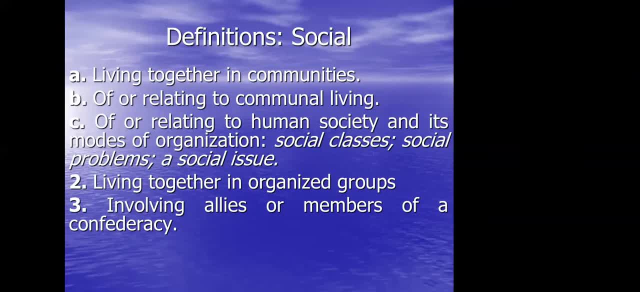 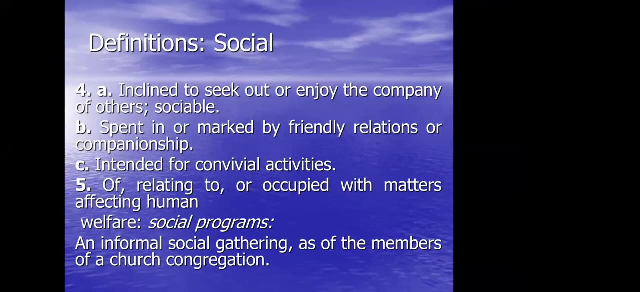 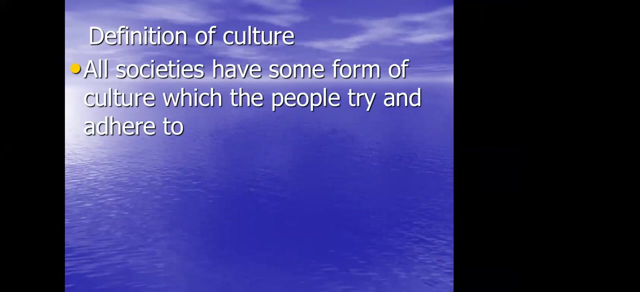 so that communal living in a society is very important. so it's living together in organized groups involving allies or member of a confederacy. so there are different definitions. we will not go through all of them. and then, as i have said, all societies have a culture. 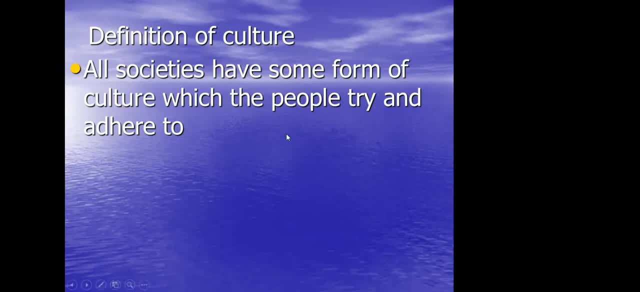 and that culture, which societies have, has a bearing on water resources. in the african context, we know that our cultures, we have a culture, we have the system of, like rain, making ceremonies. when it's like this time of the year, some communities actually gather and have those ceremonies. 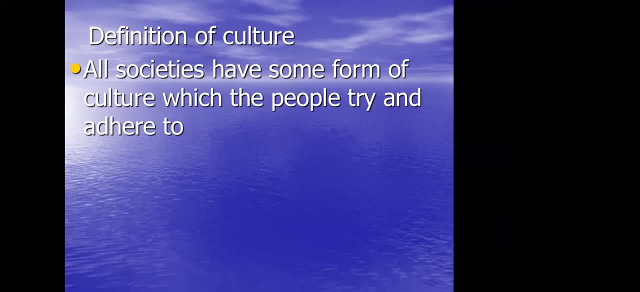 others, they actually have sacred places, which includes water sources. so all societies have some form of culture which people try and adhere to, and it's very important to know that all cultures touch one way or the other on water resources. you talk of christianity and we talk of baptism. 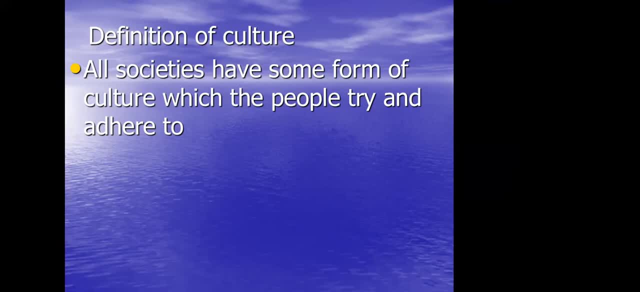 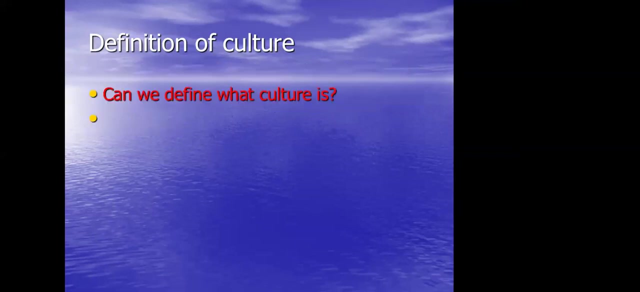 and you can't have baptism without water. even in the muslim, even you know all religions- there is water involved somewhere somehow. so what is culture? can someone define culture for us? can someone please define culture for us? culture is hello. yes, can you hear me? 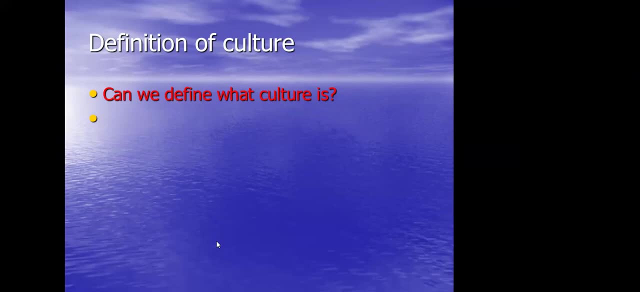 can you speak up, please, or go closer to your mic? yes, so i was saying culture is a way of living or the belief systems that people have that guide the way they live. thank you. any other definition of culture. what i can say is this: it is the idea. 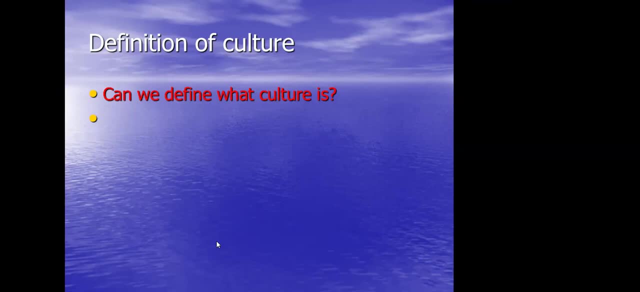 customs and social behavior of a particular people or a society. okay, thank you, that is very correct. that is very correct. yes, oh, my slide, my slide is refusing to move. i don't know what's the problem. okay, so when we are talking of about culture, those beliefs, those customs and so forth, 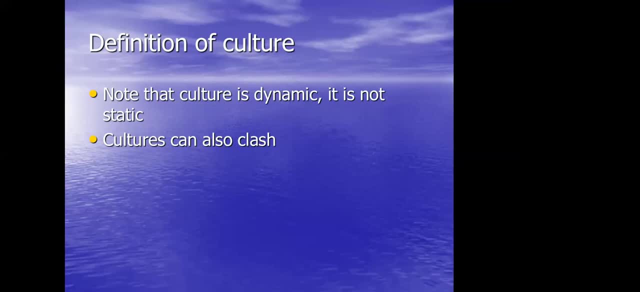 they are not static, they are dynamic and, as water resources practitioners or professionals, we need to understand how they change those beliefs, those customs related to water resources management and also cultures can clash, you see, you can go into a community and you bring in your culture. you see, maybe due to migration and so forth, 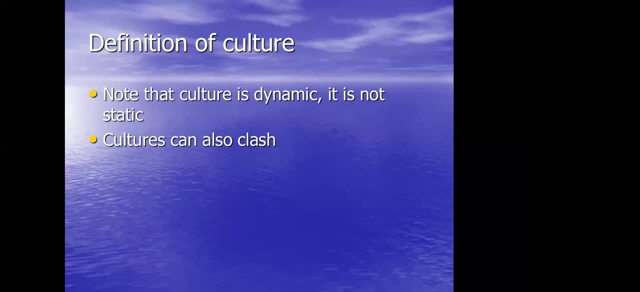 one group can go into another group and then they are. they bring their own culture and their culture will clash with the culture that is dominant within that community. so when that happens, as a water resources management practitioner, you should know how to handle it. you should know how to deal with the, with the different. 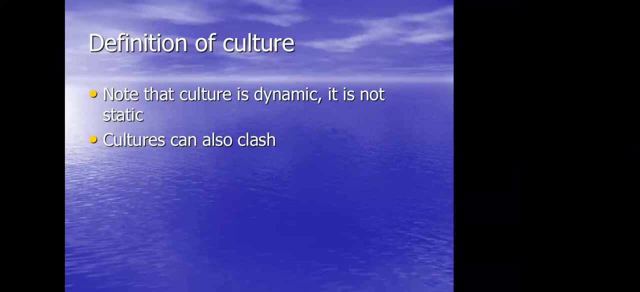 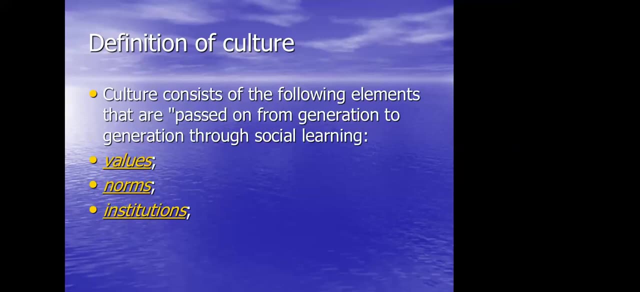 the clashes that will be taking place, uh, between or amongst the the different cultures. so culture, it consists of three elements, which are passed from us from generation, from one generation to the other, mainly through social learning. you have values, you have your norms, and then you have institutions. 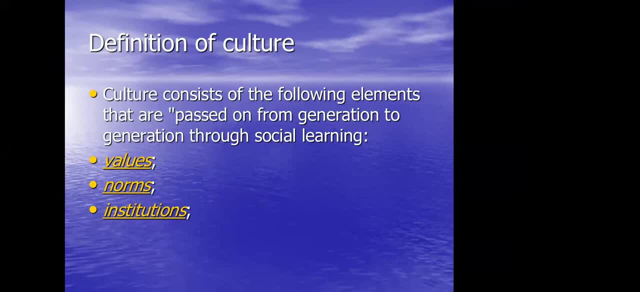 these are the most important. you know elements of culture. so when you are in a community, when you are in a society as a water resources manager or a manager- or manager is- you need to understand the values, you need to understand the norms and the institutions related to water resources management. 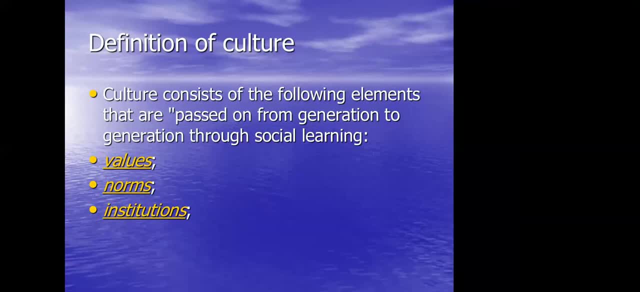 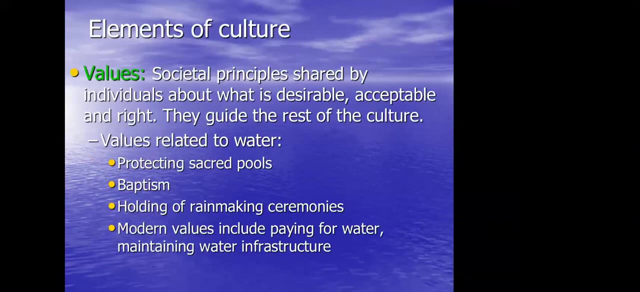 or how their values, how their norms affect water resources management, or they are affected by water resources management, or laws which may come and so forth. it is very, it is very important. so what are values? values: these are society principles shared by individuals about what is desirable, acceptable and right. 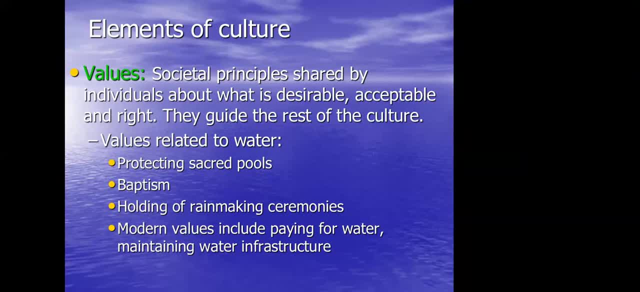 these they guide the rest of culture. so most cultures they have values related to water. the most important value is that all cultures they value water, because water is is important. so you might have values related to sacred pools, values related to baptism, values related to ceremonies, rain making ceremonies. 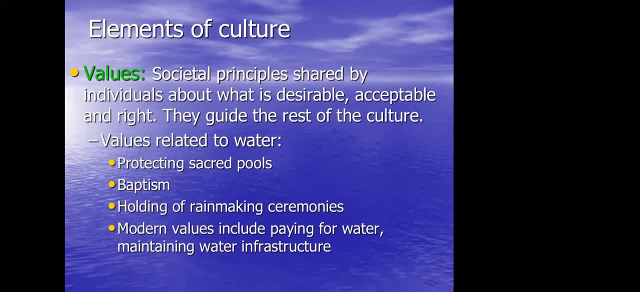 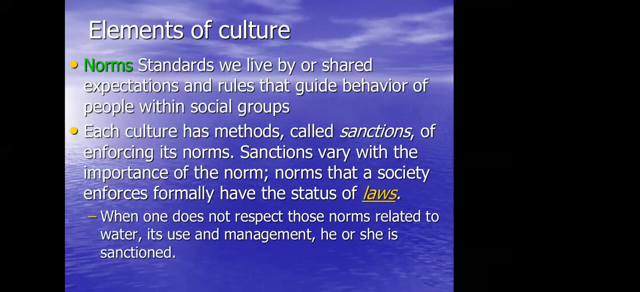 and then modern values. we are talking about water being an economic good that everyone. if you are using water somehow, you should pay for it. we are. we are putting your value on the water, on the, on the resource. and then what are norms? these are basically the standards we live by. 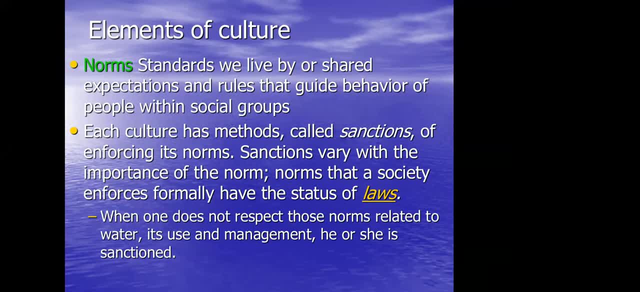 or shared expect, expectations and rules that guide behavior of people within social groups. what are the rules related to uh, related to the water resources within a community, related to those uh pools which are sacred uh sacred places, you see. so each culture has methods called sanctions. these sanctions, they now enforce norms. 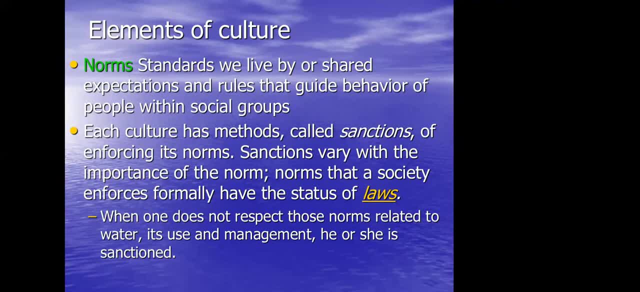 when you, uh, when someone does something which goes against or you break a norm, you are sanctioned. and some, some of the sanctions, uh, some of the, the norms that a society enforces, they, they have the status of, of laws. so when some, when one does not respect those norms related to water, 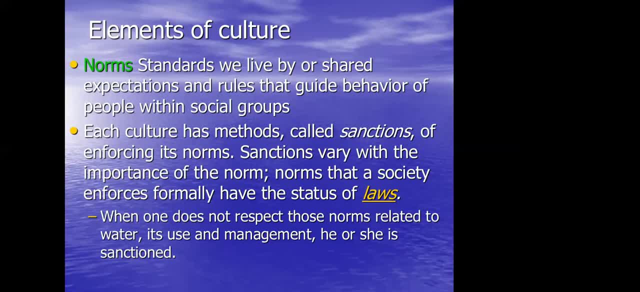 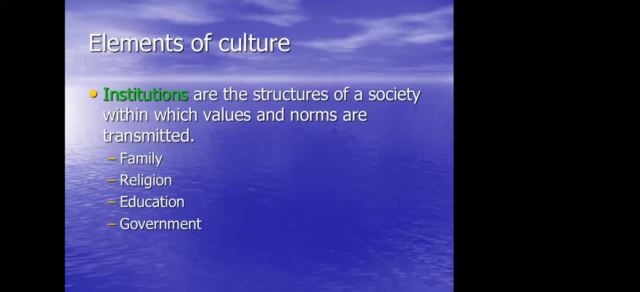 its use and management, you or she is sanctioned. and then we talk of institutions within a society. so these are the structures of a society within which values and norms are transmitted. so you talk about of the family, you talk of religion, you talk of education, you talk of the government. so 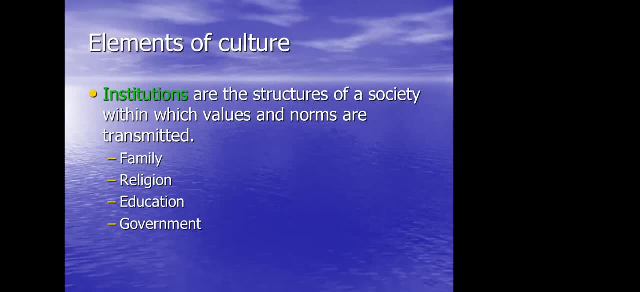 each of these institutions play their role in transmitting those values and norms. the family will transmit certain values. the religion would transmit certain values. the educational system, it can be formal or informal, transmit certain values. the government transmits and values the laws and so forth, the policies which governments put in place. so those are the three most important. 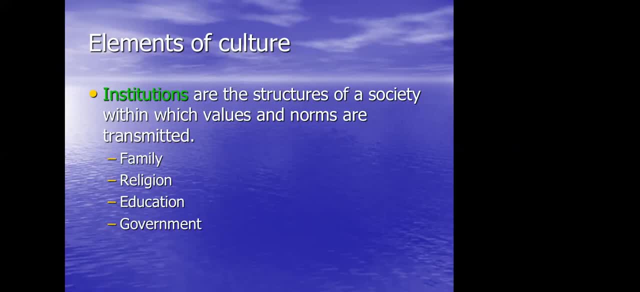 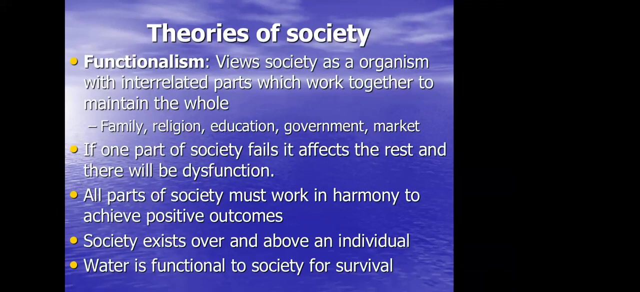 elements of culture. do we have uh questions or do we have additions on what society is, on uh culture and and and its elements. any questions or any comments? okay, so when? when we look at society, we can look at society from different viewpoints. we have abstract ways of explaining what happens. 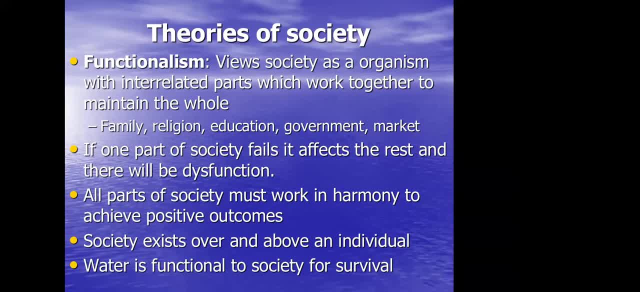 in society. so this is where we have different theories of society of explaining. it could be your culture, you see, of explaining culture, of explaining how a particular society manages its water. so we have different theories which we can, which we can use one of the theories which we 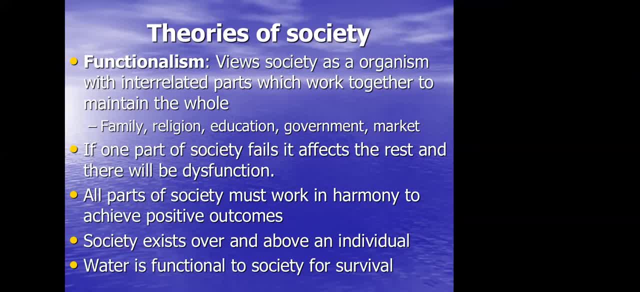 is which we can use in explaining water resources management or in managing water is called functionalism. some of you who are from like engineering field and so forth, you use models- may be hydrological uh models. you are basically trying to explain. you know a particular catchment. this is how it behaves, so it can give you the opportunity to summarize all these things. that is how we are in it's way of telling a uncut 몰�ad Tischler: the objective of undecl icing and analysis, doing any intervention. so. but you can use some of this values which we can use in explaining water resources management or in managing water is called functionalism. some of you who are from engineering field and so forth, you use models, maybe hydrological models. you are basically trying to explain a particular catchment. this is how it behaves. 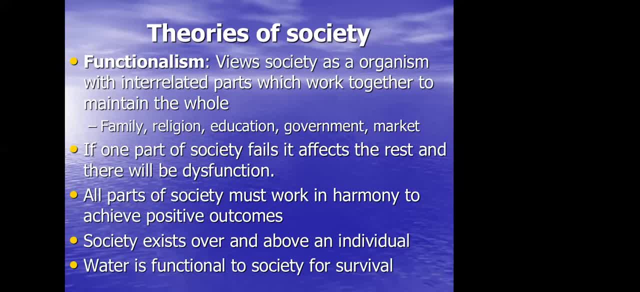 So in sociology, when we are explaining society, we use theories and say this is how society behaves, And one of the theories is called functionalism. Functionalism basically views society as an organism with interrelated parts. So they are saying society is like a human being. 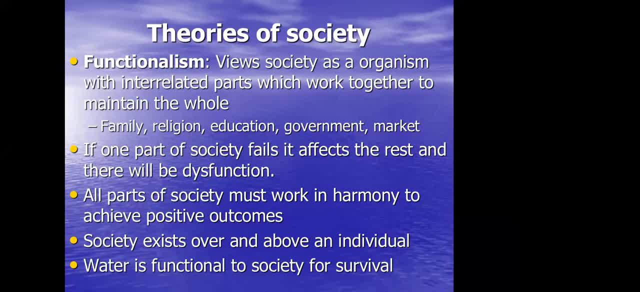 The way I am. I am made of different parts, but which are interrelated: My arms, my legs, my head, my heart and so forth. they are interrelated. If one part is affected, the whole part is then affected. 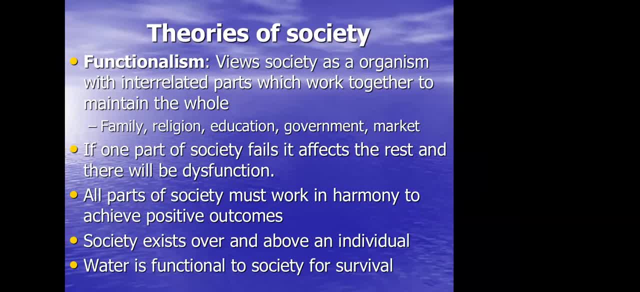 So if we really want to efficiently manage water resources, all the interrelated parts of the society, the family, there is some water resources management which happens at that level. It has to be linked to our religious system, It has to be linked to our education system, to our government, to our marketing system. 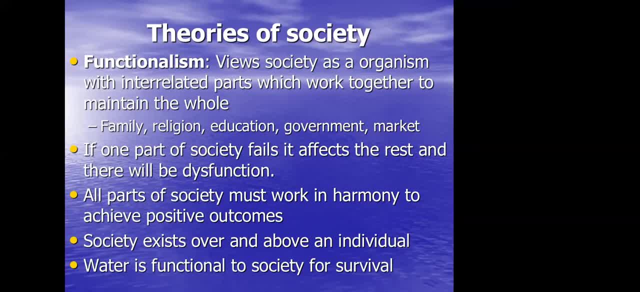 So they are saying if one part of the system fails, the whole system is affected. You see, If the government fails, the system is affected. If the government fails, the system is affected. The system is affected, The whole system is affected. 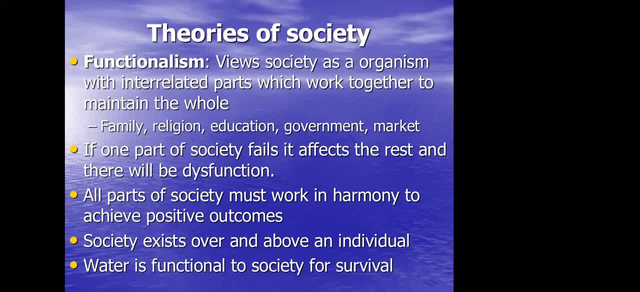 The laws, the policies and so forth. We are going to be the water distribution system, the institutions which are supposed to supply water to us. if they fail, then the whole system is affected. You see, If at the family level we are not playing our part, we are not paying for the water. 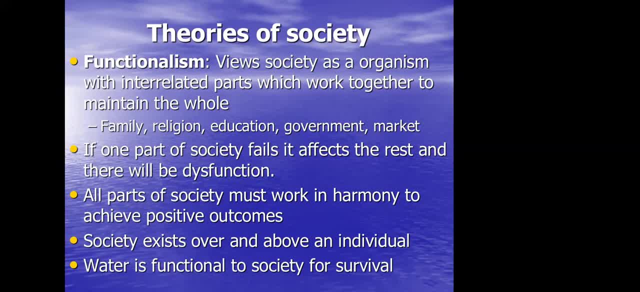 resources that we are receiving. If, at the family level, we are not doing our part, we are not investing in the water materials. You see? So this is the functionalist theory. Can we unmute our mics please? So what they are saying is that all parts of society must work in harmony to achieve 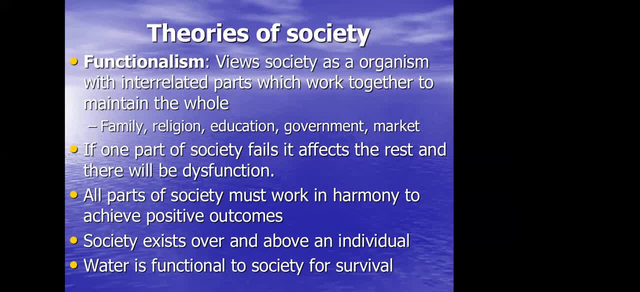 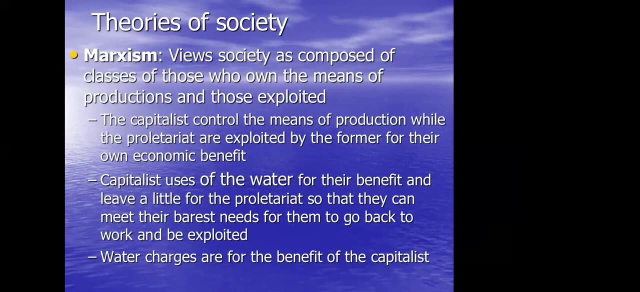 positive outcomes. That's basically what the functionalists are saying. This is a theory which was propounded by a man called Emil Dekem, And then there is a theory also which was propounded by a man called Karl Marx. This is Marxism. 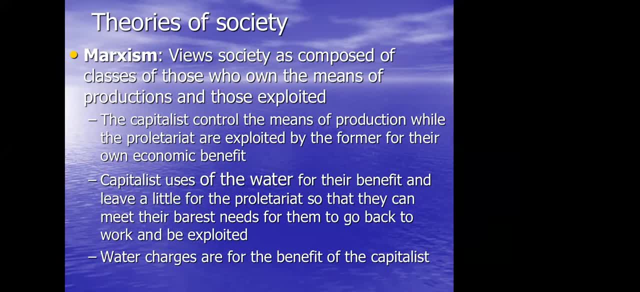 So Marx basically views society as composed of two different classes: owners of the means of production, that is, the upper class, and what he calls the lower class, the proletariats, the people who are exploited by the owners of the means of production. 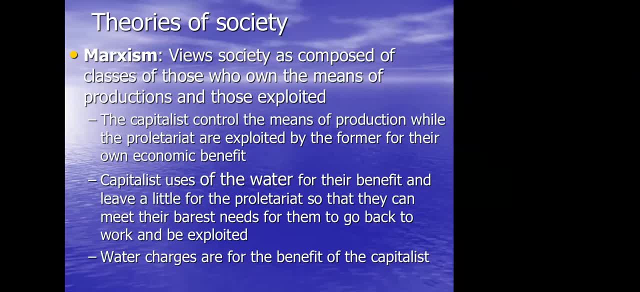 So he is saying, in society, those who have a bigger share of the water resources management, those who are using much of the productive water resources management, those who are exploiting the water resources management, they are the top people in society, They have the resources. 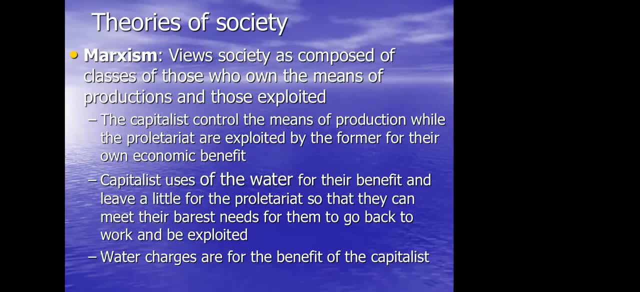 They can amass land, They can pay for the water resources And the others will just be there to work for these people. So Marx is basically saying capitalists use the water for their benefit and live little for the proletariat. So Marx is saying: capitalists use the water for their benefit and live little for the proletariat. 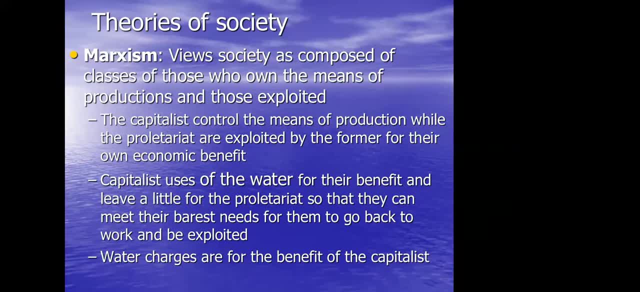 So Marx is saying: capitalists use the water for their benefit and live little for the proletariat So that they can meet their barest needs, for them to go back to work And also the issue of paying for the water resources. Marx is saying: when you put charges, 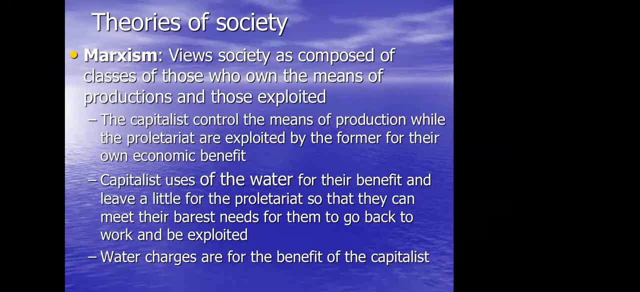 on water, you see only those with the money, with the resource they can use it, and the people who are able to use the water. That is why you see governments coming in with pro-poor policies, so that no one is denied. 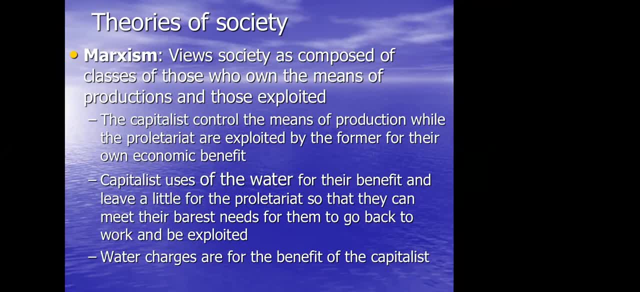 the right to water. You look at governments like South Africa and so forth. they actually have a certain amount of water which is available for free to a household. It used to be about six cubic of water. I'm not sure if they have revised that. 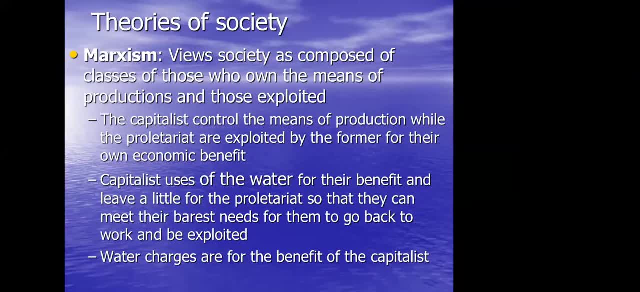 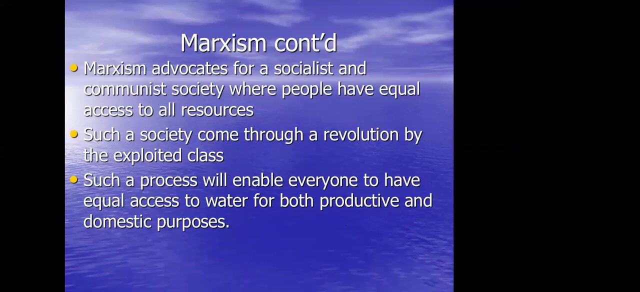 So the first six cubic meters of water that you consume is for free. They are trying to close the gap between those with the resources and those who are poor. And then Marx, of course, advocates for a socialist society, Socialist, communist society, where everyone is able to equitably access all the resources. 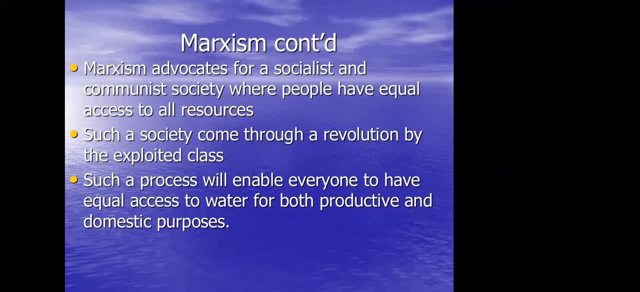 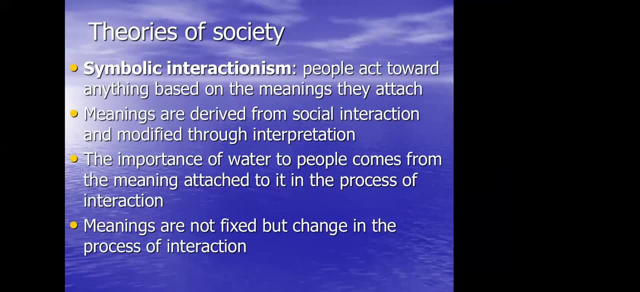 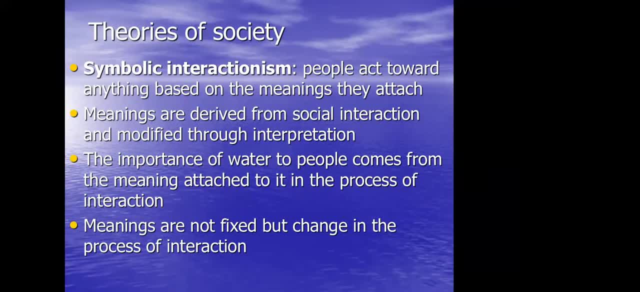 Symbolic democracy, Symbolic interactionism, Symbolic interactionism. This basically denies the notion of society as given by Marxists and as given by the functionalists. It says society is just composed, doesn't have a culture, it's just composed of individuals. 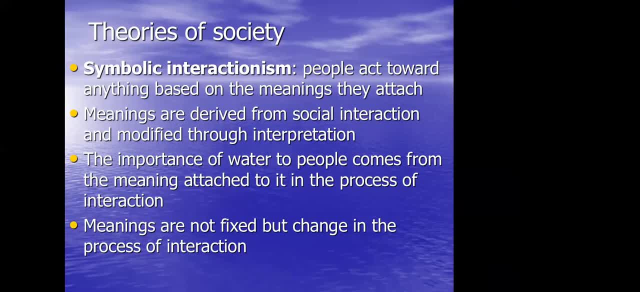 Who acts towards anything based on the meaning that they attach. If you attach a meaning saying that water is important in your society or in your community, or to you as an individual, then you will put in place measures to protect it, to enhance its management. 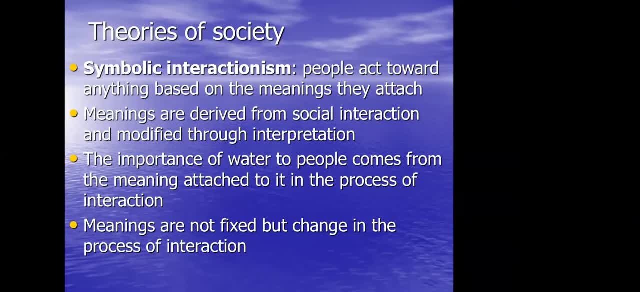 So, whatever you do to your water resources management, it depends on the meaning that you attach. If you think that water is not important, then you will not attach any meaning to it. you will not put in place measures to manage. you will not put in place any institutions. 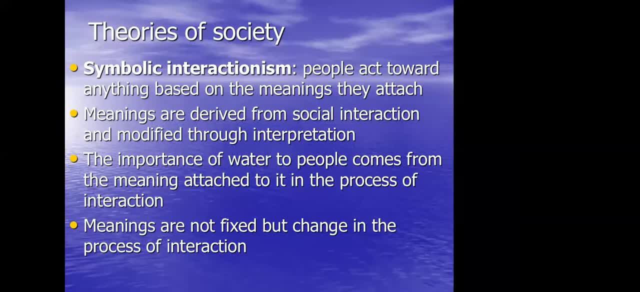 to manage the water resources. So they are saying meanings are not fixed but they change in the process of interaction. As you progress in your particular context your meaning to water resources management can change. You might have pollution coming in because you are no longer attaching. 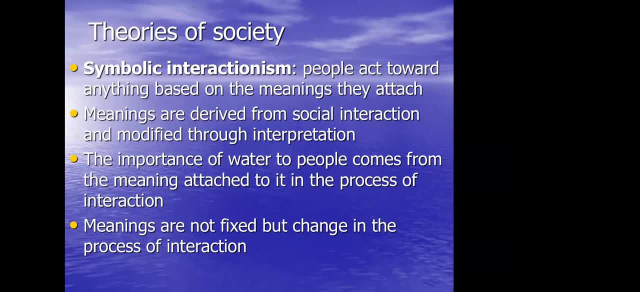 an important meaning to the water resources. So it's just like the just ended COP conference has been trying to do. We're using it as symbolic interaction is interpretation. We are saying the world is putting an important meaning on climate And because they are putting an important meaning on climate, 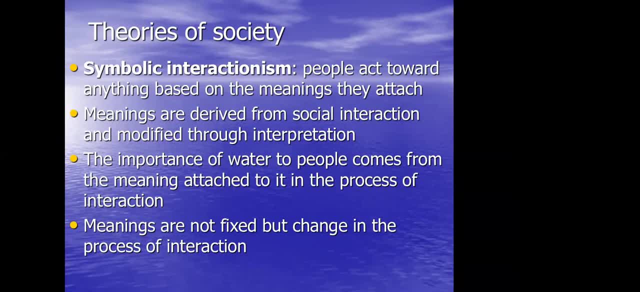 they are now. the world is now trying to put in measures to ensure that our climate is not negatively, our earth is not negatively affected by climate change. It's all about the meaning that we are putting on things. So that is the symbolic interactionist theory. 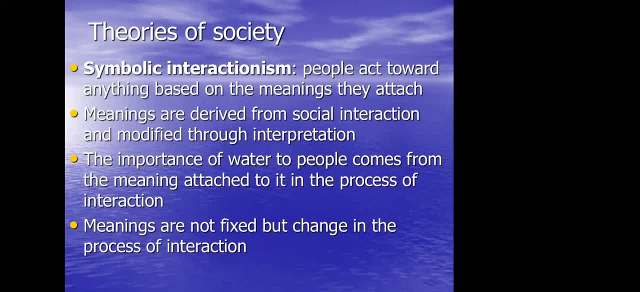 I don't know if we have any questions based on the three theories that I've presented. Thank you, Are we understanding any comments in the chat box? I'm not seeing comments. Okay, I'm just seeing someone who was defining what society is. 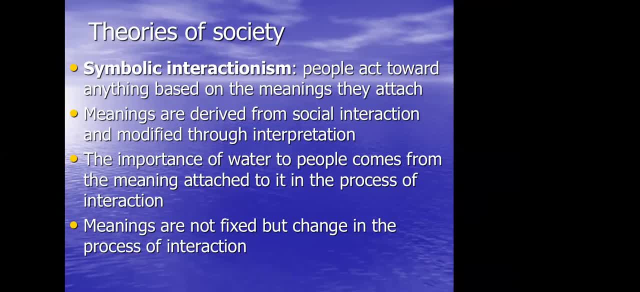 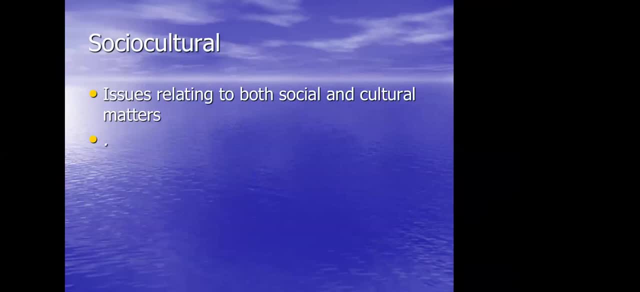 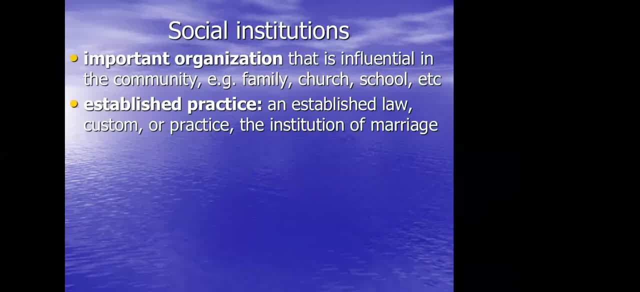 we are talking about issues relating to both social and the cultural matters. So socio-cultural institutions, we then put in place institutions that are influential in the community. You see, even for water resources management, for even our laws, customs and practices. 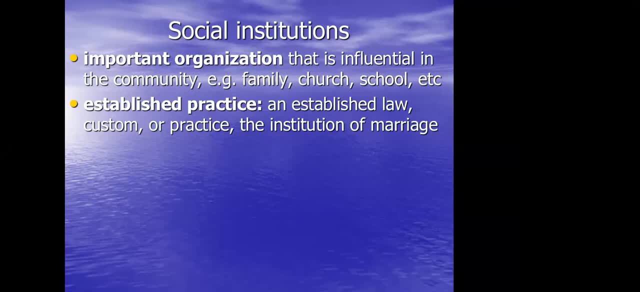 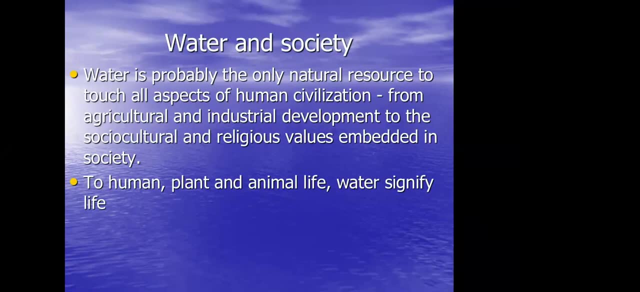 that our water resources are managed efficiently. So when we now look at water and society, we see that water is probably the only natural resource to touch all aspects of human civilization, from agriculture, industrial development to the social, cultural and religious values. 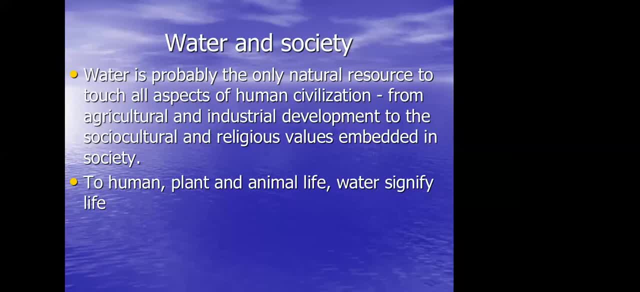 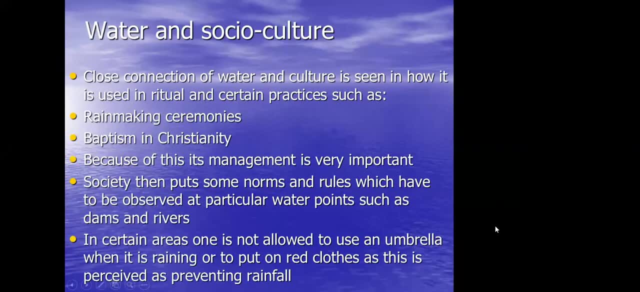 embedded in society. to human, plant and animal life, Water is very important, So close connection of water and culture is seen at how it is used in rituals and certain practices such as rainmaking ceremonies, baptism in Christianity. because of this, its management becomes very important. 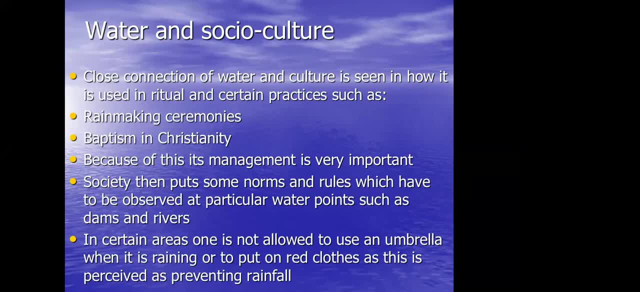 Society then puts in some norms and rules which have to be observed at particular water points, such as dams and rivers. You see, so there are. if we look within our societies, there are certain norms that we have related to water. Don't do this. don't use an umbrella when it's raining. 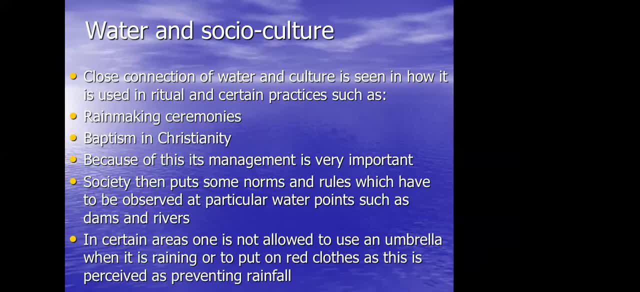 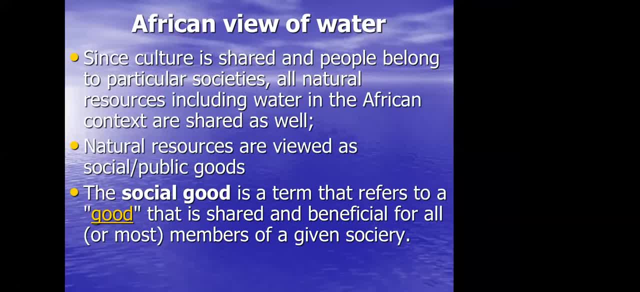 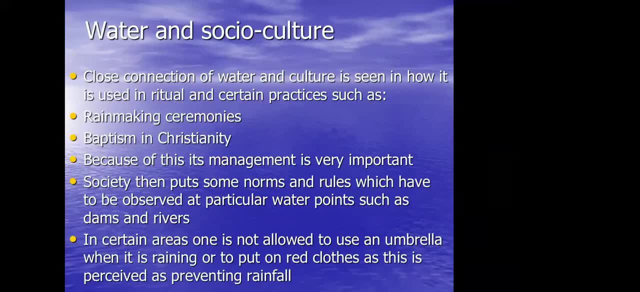 Maybe you can give us some examples from your different culture, from your different cultures or from your different societies, of certain norms or certain rules that pertain to water, Be it rainwater, be it rainmaking ceremonies, be it. what can we? can we have examples from our 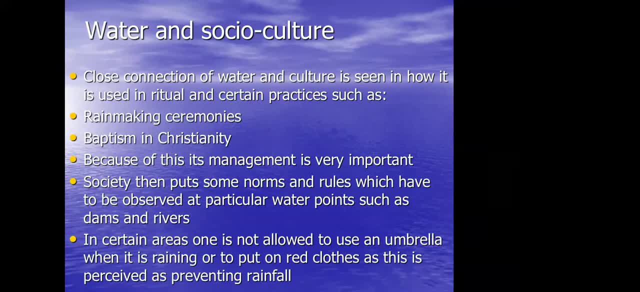 from your different contexts. Anyone, Hello, Any examples please? Can we please have some examples? Are people still there or I'm talking to myself? Can someone confirm that I'm still in the meeting? We are here, doc. Okay, okay. 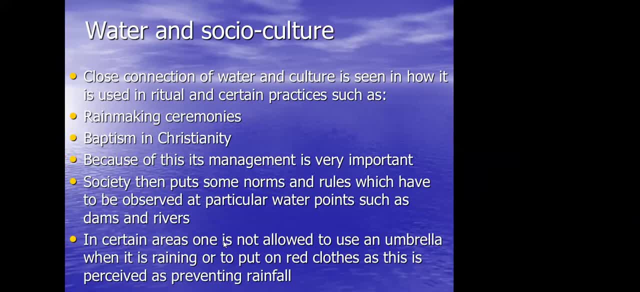 We are still in the meeting. Okay, can you speak up please? Okay, Mindu Mindu, you can unmute um? culturally, people say that uh, just to mean that uh, water is viewed as being clean regardless of the source. okay, yes, thank you. any other intervention? 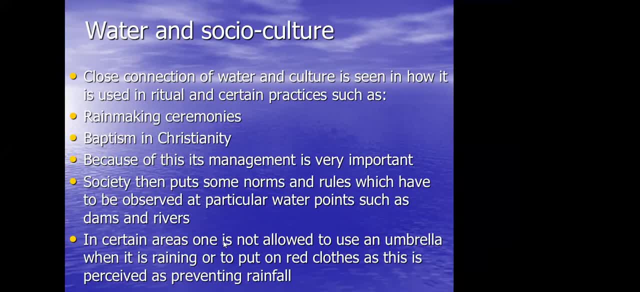 um culturally in mutoko, or the people from that area. the first thing that is done when you get to their homes, you are given water to drink. yes, signifying life. they are sort of celebrating, you know, uh, life, you know, and also that we are all somehow. 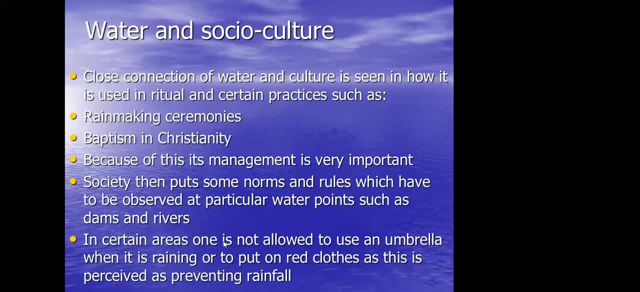 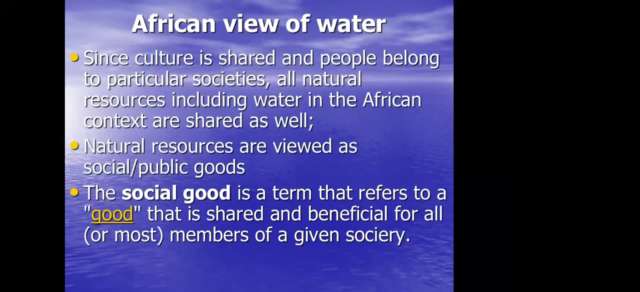 are linked together, you know, by with water. okay, any other intervention, okay, thank you. so since culture is uh is is shared and people belong to a particular society, all natural resources, including water, in the cultural uh, in the african context, are shared as well. natural resources are viewed as social or public. 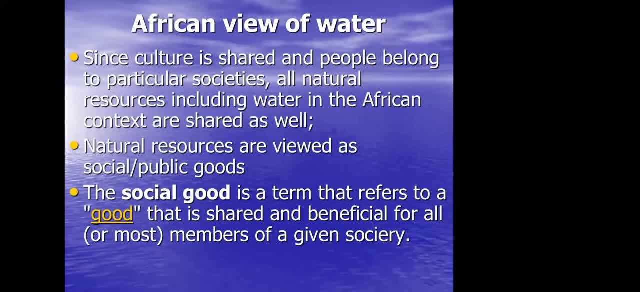 goods. the social good is a term that refers to a good that is shared and beneficial for all, or most, members of a given society. so this is what most african cultures, uh, say. this is what they share in common: the resources that we have. these they come from a higher being. it could be gods. 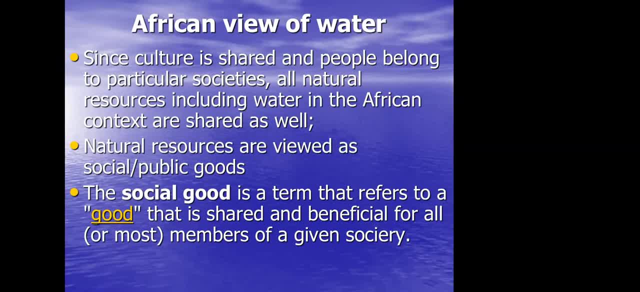 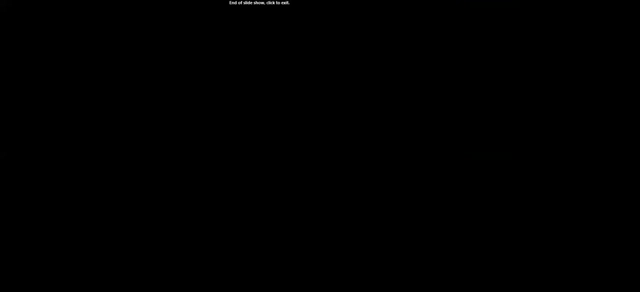 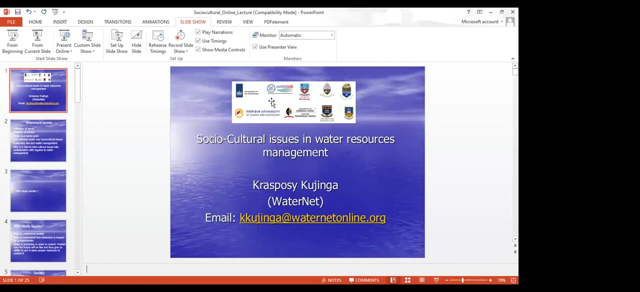 you know in uh. when you are talking in uh in christianity uh terms, you see, it could be ancestors who give us natural resources, including water, and because they are, these resources are freely given. no one should be denied access to access to the to the resource, uh, thank you. so much about socio cultural issues, but what is important is. 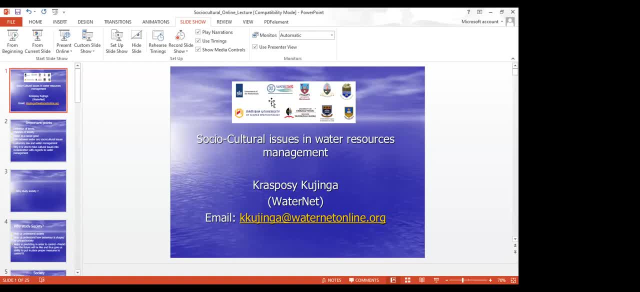 that these issues, they are very important when you are um doing any project within an african, an african context. how i mean? a culture is important, understanding society is important, understanding society is important, understanding society is important and a cultural context is so important, important. Any comments? 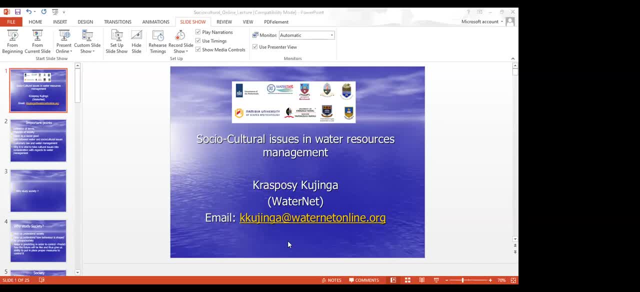 Any comments? Maybe let me see There is someone who has posted in the chat box. He's saying that's lobster. In my area they brew beer during rainmaking ceremony. Yes, this is common in most African cultures: Rainmaking ceremonies before the onset of rains or when there is. 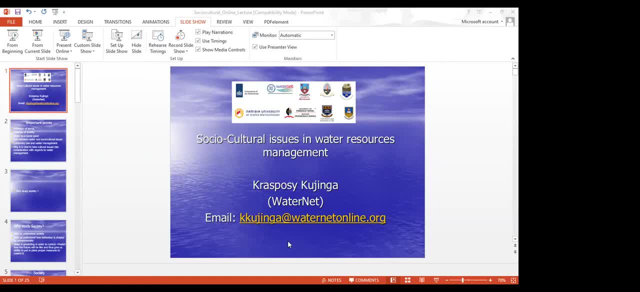 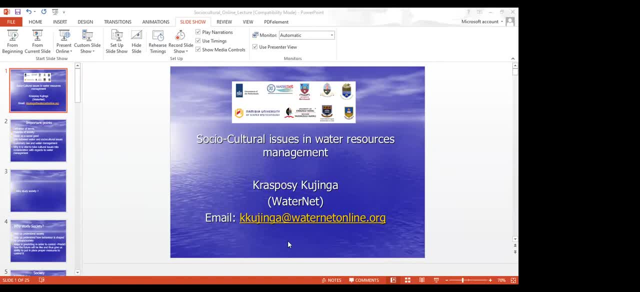 utaPlank politics. these people used to depend entirely on the Zambezi River for farming, for fishing and so forth, do regularly do these rain making ceremonies, Even when there is a drought, they would say. when there is a drought, they will set aside a particular day, they will brew their beer. 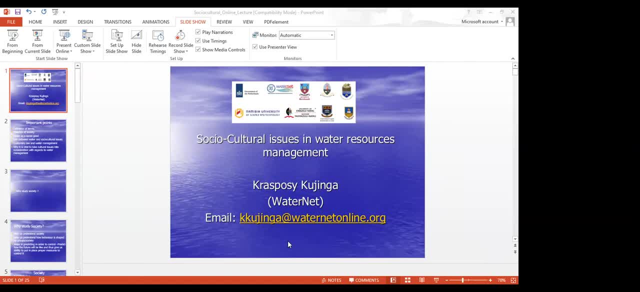 and then, on a particular day, they will go and offer the beer to the ancestors And then they say: in most cases, after performing those ceremonies, that day or that evening it will rain. You see, I don't know whether that is true or not, but that is what they say. Maybe the book? 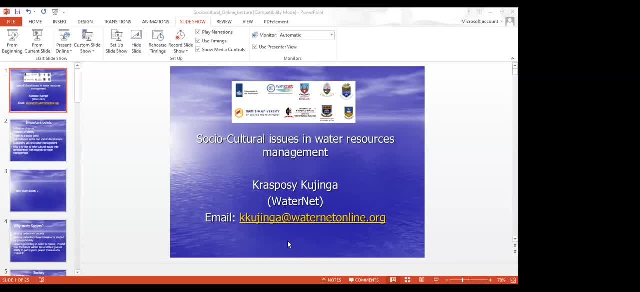 is available on the internet. If you look for a book called People of the Great River, you see it's about the Tonga people. they believed in their god, the Nyami Nyami. Now they say because of the Kariba dam wall. 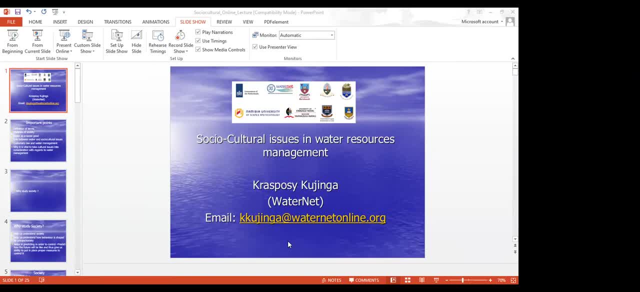 the Nyami Nyami, the female Nyami Nyami and the male Nyami Nyami were separated. The male Nyami Nyami, I'm sure they say, remained on the upper side and the female is on the lower side. So around Kariba dam they sometimes experience tremors and then they say their 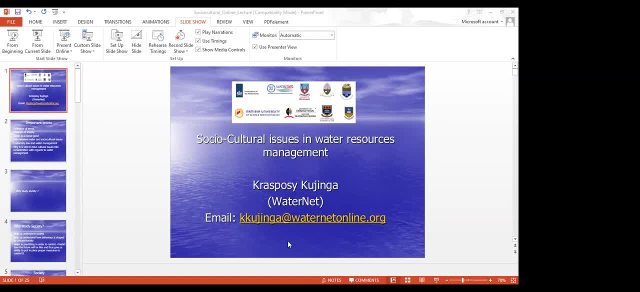 interpretation is that it is because the male Nyami Nyami wants to go to the other side, where the female Nyami Nyami lives. So that's, that's culture. So the other person? yes, in our culture, when people come back from. 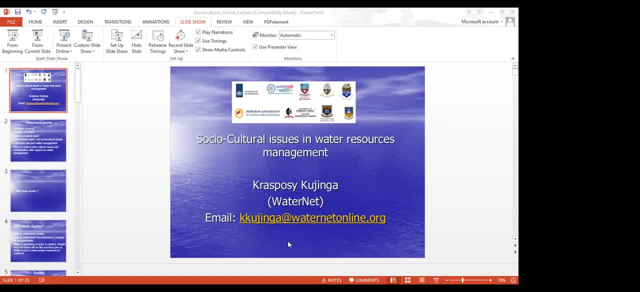 the burial, they put a dish of water at the gate for cleansing. Yes, in most cultures, water is used for cleansing. This is very true. And then then Mapanisa is saying how our cultural value is considered within the context of IW R-I-M framework. So when we are talking about society, 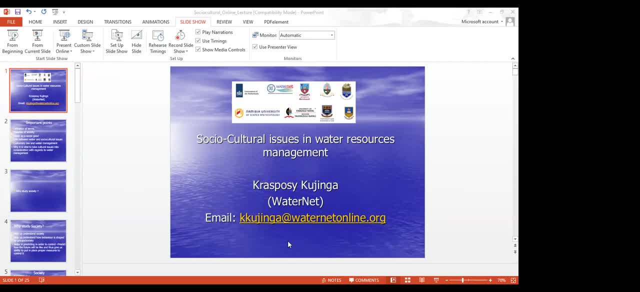 and then we talk about society as having a culture, and then we are saying: when you are managing water resources in any context, understand its cultural values, because you will not then be able to introduce other elements of IWRM. if you don't take into consideration its cultural values, your interventions can be uh resistant. I can give you an example. 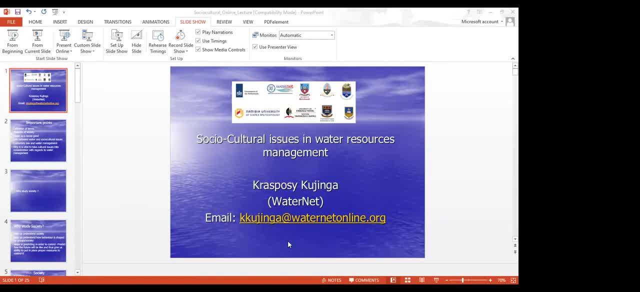 of uh, of what happened the other time in uh in Zimbabwe. uh, we have a dam called Osborne Osborne Dam, so our national water management institution is called the Zimbabwe National Water Authority and we have a dam called Osborne Osborne Dam and we have a dam called Osborne Osborne Dam. 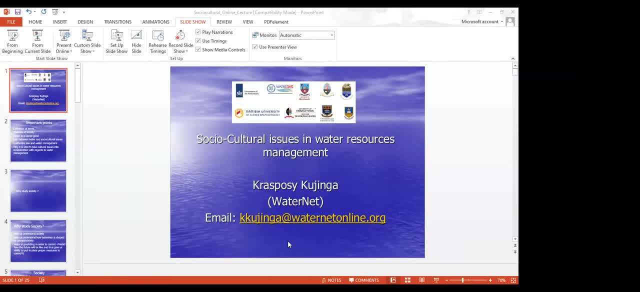 so they have a dam which they manage in this uh, in this area. so they were pumping water from that dam to um, to to the nearest city that is, uh, that is, Mutare. but what happened is that the pumps were constantly breaking down. they would replace them and then the pumps would break down. 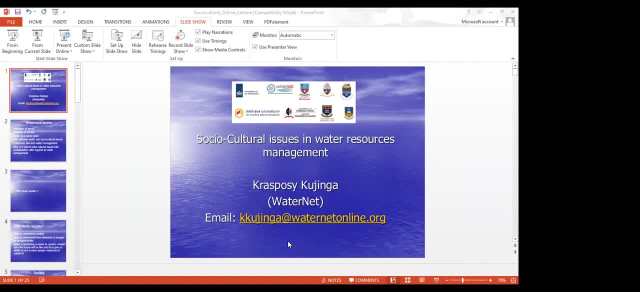 until someone, uh, advised them and say, no, this breaking down is not normal, it's not scientific. you see, you need to approach the chiefs of this area and find out what the problem is. so they approached the chiefs of that area and then the chiefs consulted the spirit mediums. and then the spirit mediums of that area, they said: 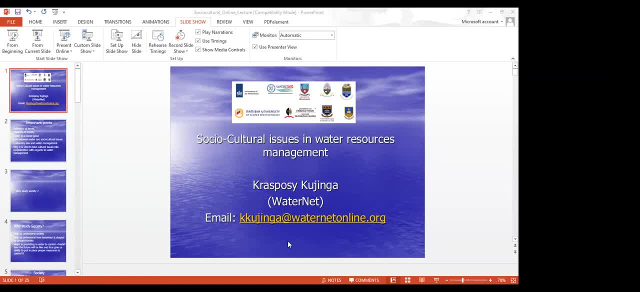 it is because when the dam was built, when the pumps were put, they were not consulted as the owners of the land. so they gave, uh, some instructions on what has to be done. they said traditional beer must be brewed, cattle must be must be slaughtered during a ceremony to cleanse the area and the authority. 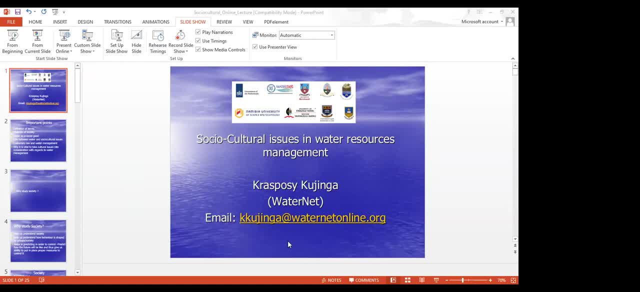 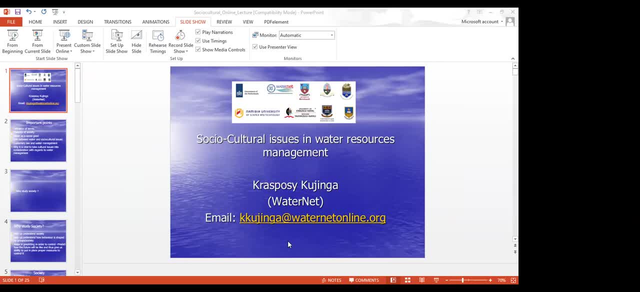 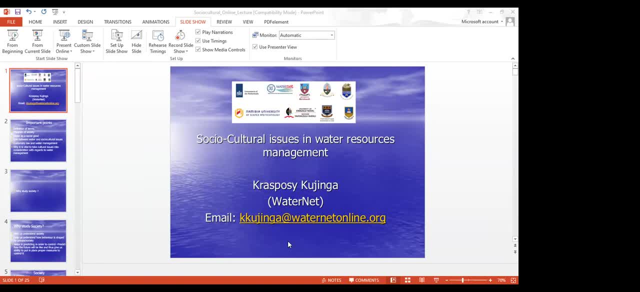 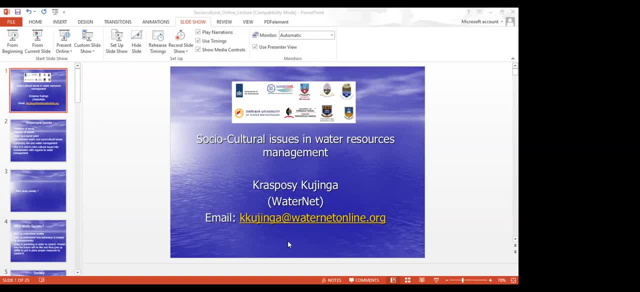 framework is taking into consideration cultural values in um in our program. iwrm framework is taking into consideration cultural values in um in our program iwrm. The elders wash first. never refuse to give water to the stranger. People wash their hands to clear conflicts. People pour water on the ground to feed the ancestors. 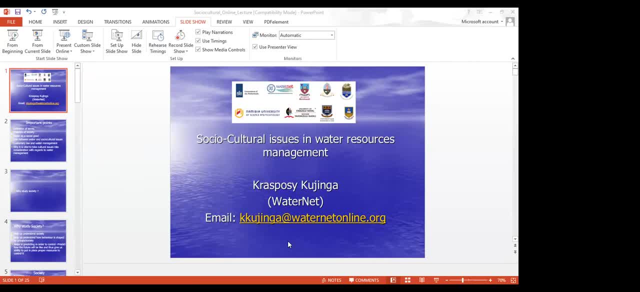 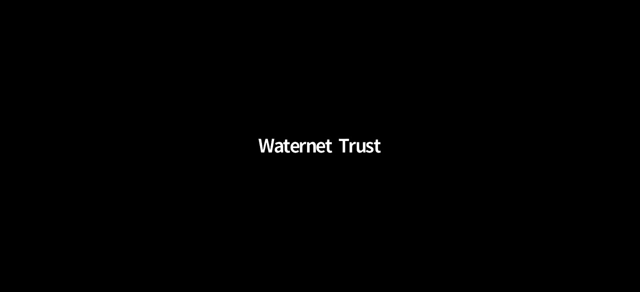 These are some of the cultural practices done in our African context, And IWRM has to take into consideration all these issues. you see, Thank you. Do we have any other comments? Any other comments? Okay, Thank you, And then our next. 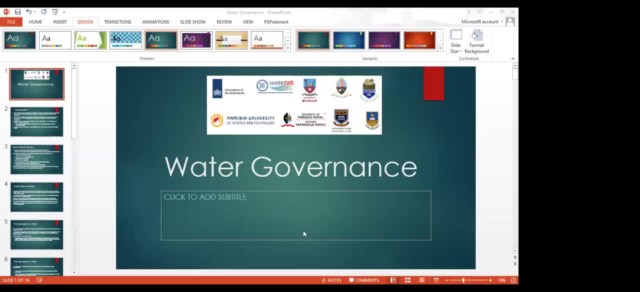 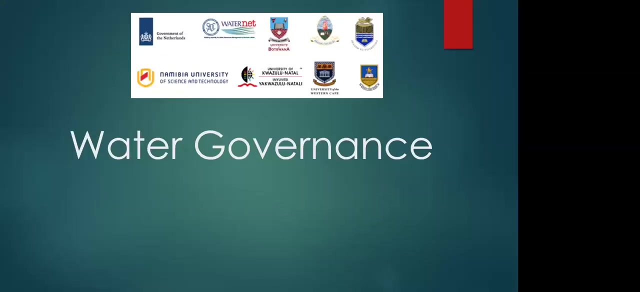 Presentation is on water governance. All right, So we want to Talk Briefly on the issue of water governance and what we have been talking about. society and culture. They are also considered within the context of water governance- how water is governed, how water resources are managed within a society, within a country or globally. 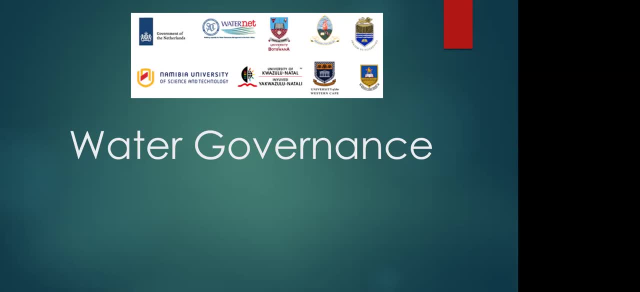 And I am taking this opportunity to ask myself, As a person that has no experience with water governance, maybe before we go into this, what do we understand by water governance? Can someone define what? what it is based on how you understand it? 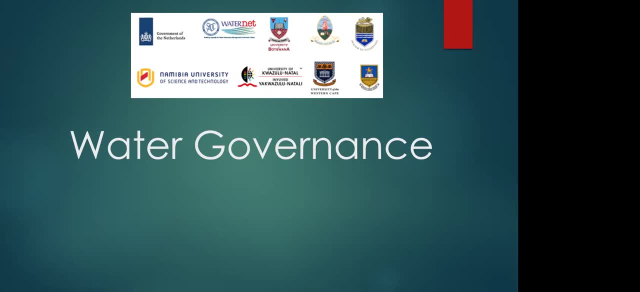 What is water governance? Anyone? Yes, Okay, Thank you. I was wondering about the work that you are doing in the context of water governance and how these work is. How do you say that is water governance And how is water governance? 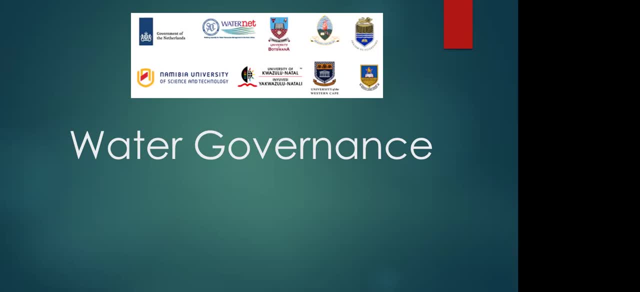 Can you tell me what the definition of water governance is And what is water governance? What do you say about how it works? Okay, Thank you. Thanks, James. Thank you, Thank you very much. Thank you, Bonjour. Thank you. 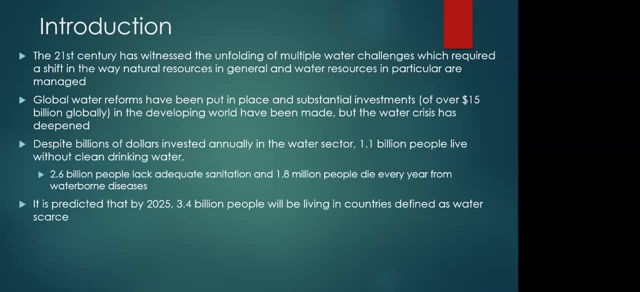 Thanks. So Anybody else? Hello Okay, Yes, Hello Yes, Go ahead, Go ahead, please. Good morning, Good morning, How are you? My name is Emerson Shambane. I am, yeah, I'm. 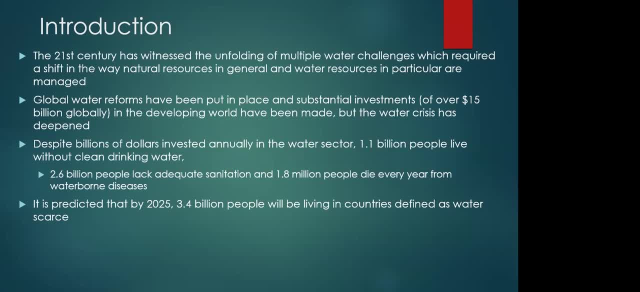 from. I'm from. can you hear me? Yes, we can hear you, Thank you. Thank you, Thank you very much Before. before you introduce: sorry, my poor, my poor English. Okay, Okay, It's fine. 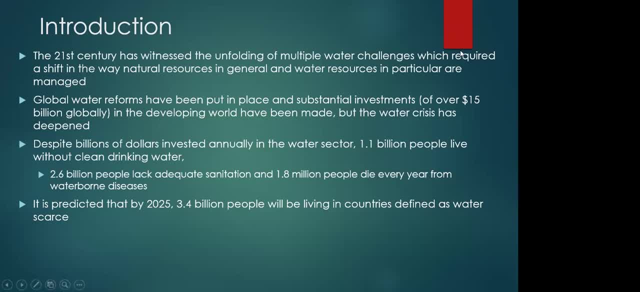 But I will try to. I will try to give me my idea Before we use some some some aspects about the presentation before of the social cultures of water. First I want to congratulate you to the presentation. The presentation was be clear for. 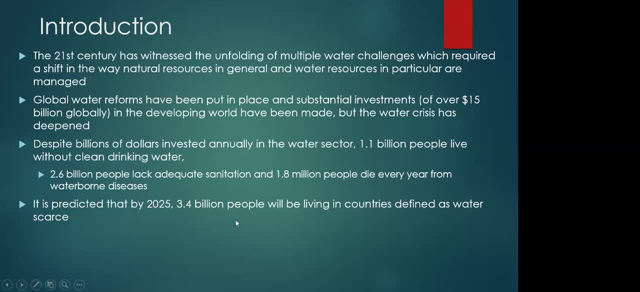 me, I think for all of us. Second, it was very important to realize this relation between culture, social and water suspects, And it's important to society In that time we see and we saw the people that use water, but there's no understanding. 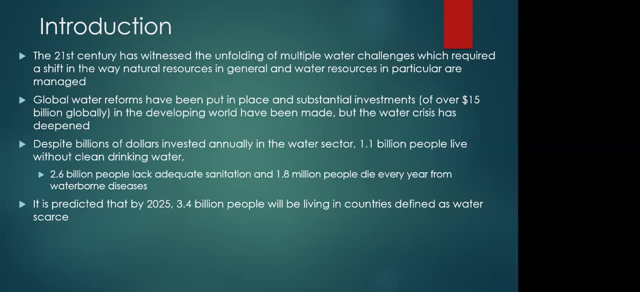 Hello, we are losing you now. It's very what the importance of water, of what the importance to use of water? We often talk about water, but we- I don't know if you can hear me. I don't know if you can hear me. 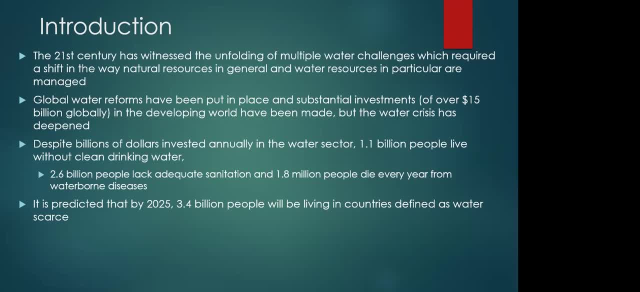 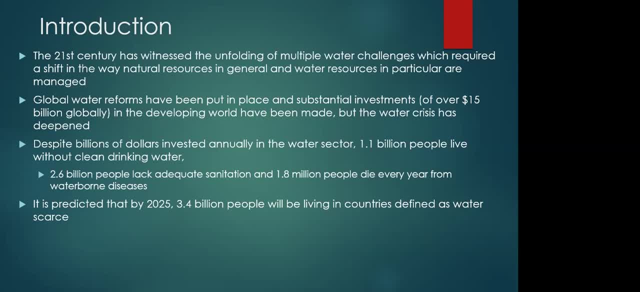 Hello, Hello, Maybe can you type. can you type in the chat: Hello, hello. Can you type in the chat box? Okay, okay, Yeah, okay, Okay, okay, I will, Okay, okay, I will type. 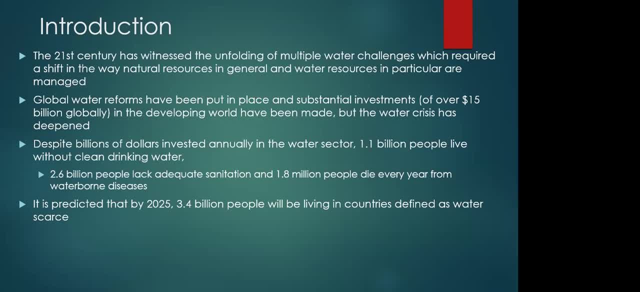 Yeah, Okay, Thank you, Thank you, you, you can come in. Thank you so much. When we are looking at water governance from my own perspective, looking at the issues like political side of the water management and the social side, 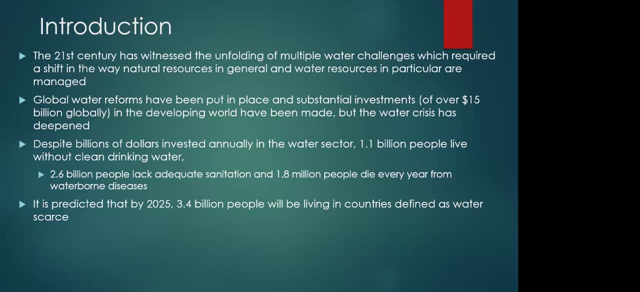 the economic management and the management system that is in place to influence water use and management. Thank you, Okay. thank you, Willard. Kindly unmute. Okay, can you hear me? Yes, we can hear you now. All right, thank you. 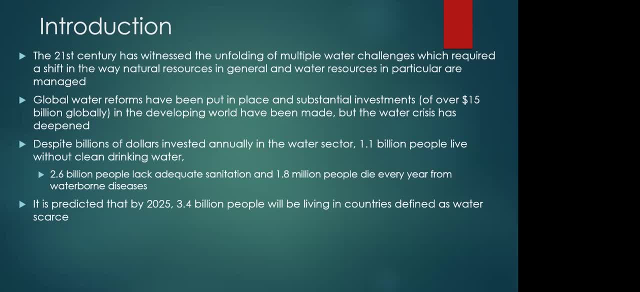 I think the response was just similar to the previous speaker. it's basically the political, social, economic and administrative systems that influence water use and management. Thank you, Okay, yeah, Thank you. Thank you. Who else? Emerson, do you want to say something? 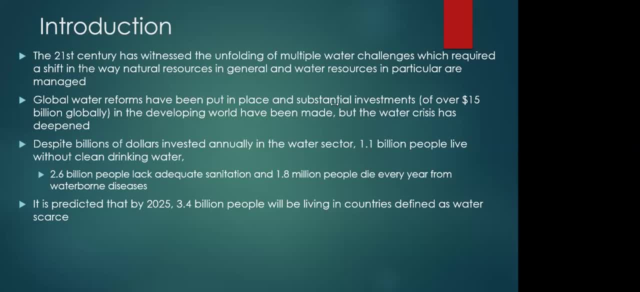 You are unmuted yourself. Yes, I Okay. okay, Kindly unmute. sorry, I unmuted you, Emerson. Okay, Paul, do you want to say something? Okay, I don't know what happened to Emerson. Emerson, kindly unmute. 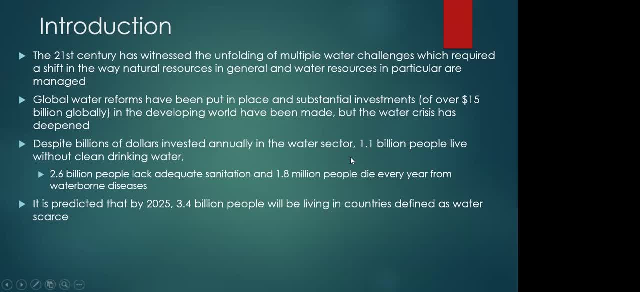 You can hear me now. Yes, we can hear you. Sorry, I think my internet is very unstable, Sorry for that. Okay, I was saying that it's very important to realize this relation between cultures, sources and water species, And it's very important to source it. 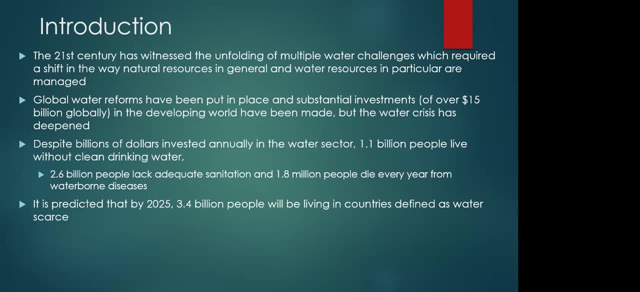 We often talk about the water but we ignore some aspects related to all ethnic origins. We often see some unprotected water sources, Sometimes because we don't understand, we don't see. it's very important. It's very important to this relation between social culture and the water. 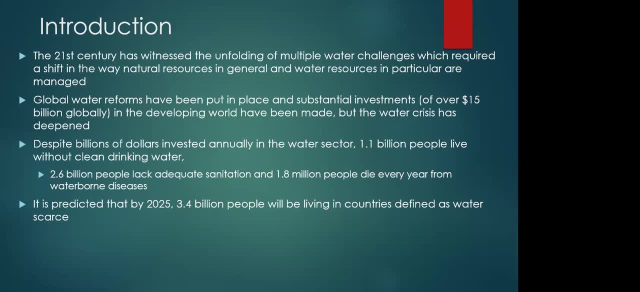 In this aspect. it's very important to another how to say to water governance, Because the water governance will do it, the direction, how to other people use the water. Is this my opinion? Sorry again for my poor English. Okay, Thank you very much. 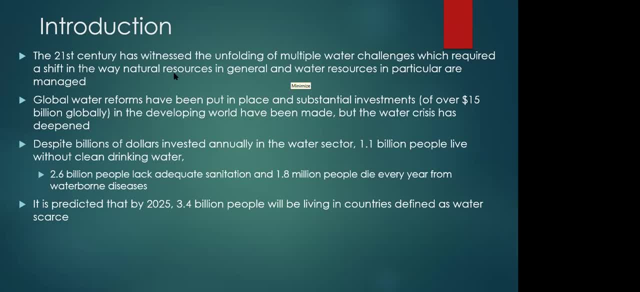 Okay, Okay, Thank you very much. Yeah, Actually, going back to culture, you want to improve water management within a particular community or within a particular society. Understand How they are currently managing the resources. So you start from that point. 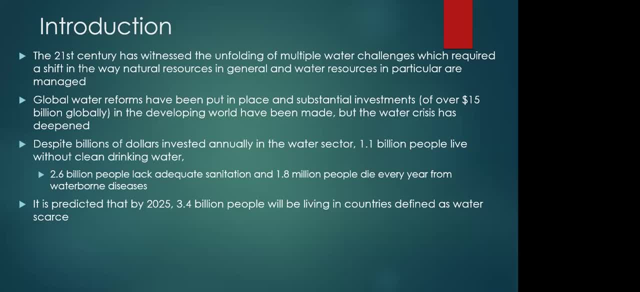 You don't come in with your own ideas and try and impose them on their culture. First understand their systems and then you can then build, you know, on what will currently be happening in there in that particular particular context. Okay, 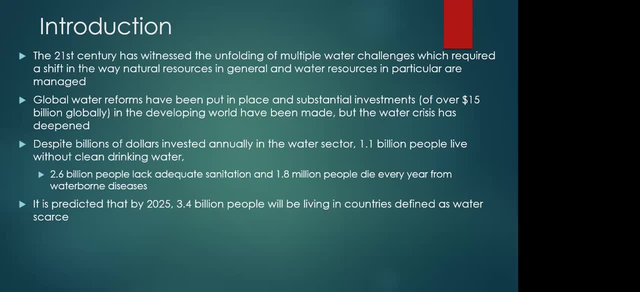 Thank you. So now go into the into into the broader issue of water governance. So maybe the first thing to notice that the 21st century is actually witnessed the unfolding of multiple water challenges, which required the shift in the way natural resources in the 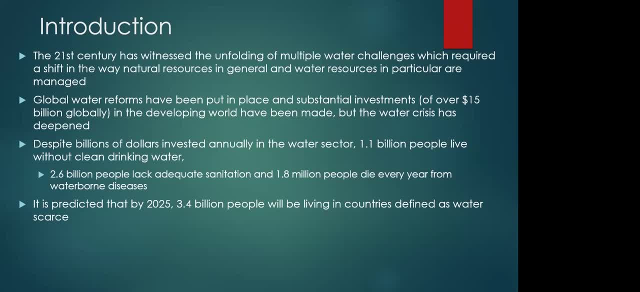 in general and water resources in particular are managed. I'm sure yesterday, Mr Kumindo-Gadeo, we have been talking about the effect being more of sectoral management of water resources, you see, And because of that, challenges started emerging. 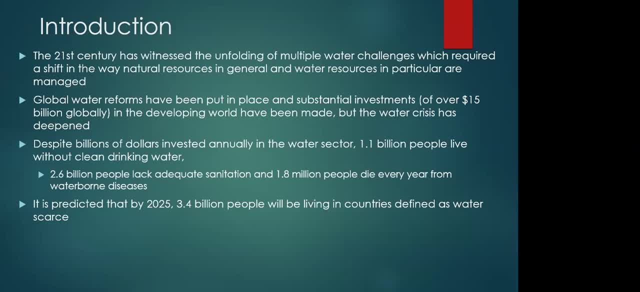 You had, for example, people from agriculture managing water on their own, people from industry on their own, people maybe from the energy sector on their own. So that was sort of sectoral management. So global water reforms have been put in place and substantial investments of over $15 billion. 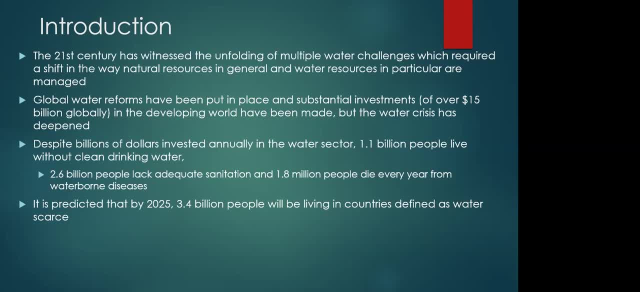 globally, in the development world have been made, But the water crisis has deepened. So, despite the billions of dollars invested annually in the water sector, 1.1 billion people live without clean drinking water. 2.6 billion people lack adequate sanitation. 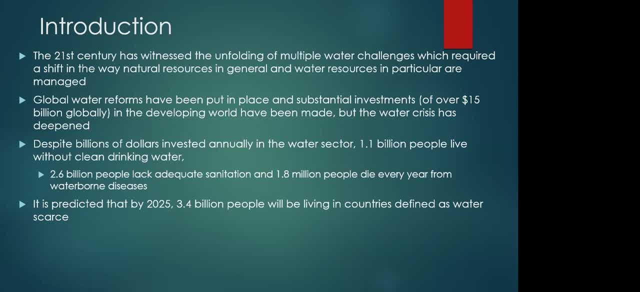 and 1.8 million people die every year from waterborne diseases. It's predicted that by 2025, just a few years, just a few years from now- 3.4 billion people will be living in countries defined as water scarce. 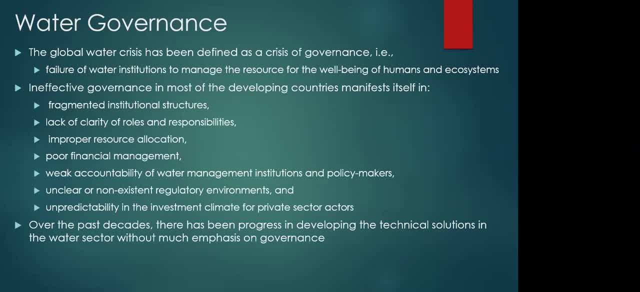 So this global water crisis that we are currently facing has been defined as a crisis of governance. It's not that the argument is that. it's not that. It's not that the government is not fighting for the economy: There is not enough water. 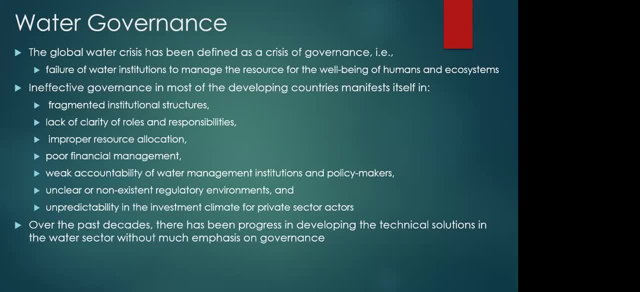 It's just failure of water institutions to manage the water resources for the well-being of human ecosystems. I can give you an example of South Africa. We have this amazing basin shared by eight countries. You know that only 14% of the water within the region. 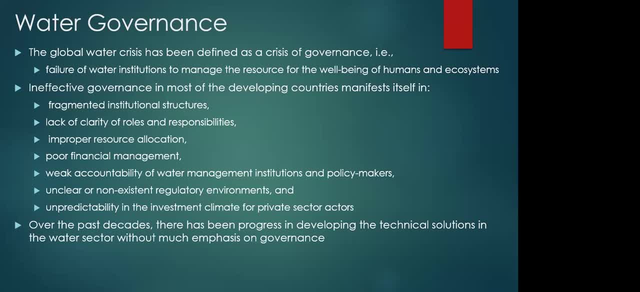 you know, within the Zambezi Basin is developed. Developed meaning that it's deemed we can use that water resources. Where is the rest of the water going? you see, So ineffective governance in most of the developing countries manifests itself in one fragmented institutional structures. 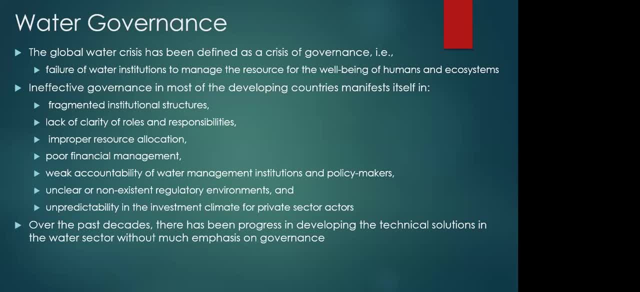 lack of clarity of roles and responsibilities, improper resource allocation, poor financial management, weak accountability of water management institutions and policy makers, unclear or non-existent regulatory environments and unpredictability in the investment climate for private sector actors. So over the past decades, there has been progress. 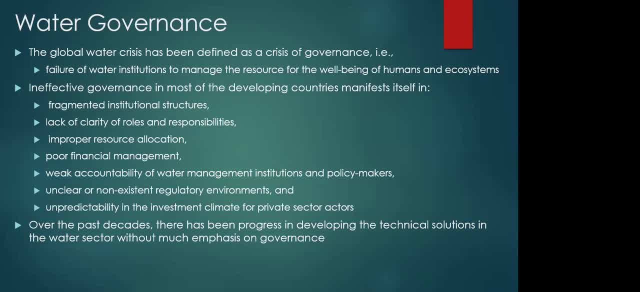 in developing the technical solutions in the water sector without much emphasis on governance. So there hasn't been a balance. you know technical and governance And our governments also. they are not really putting in you know adequate resources and also the policies. 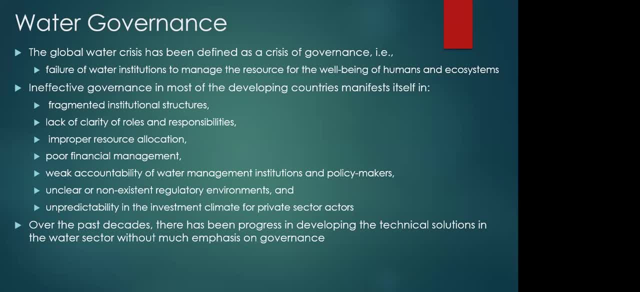 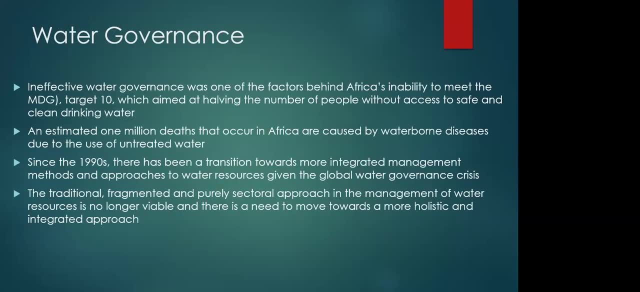 and the institutions which can really enhance governance. So the balance is not there. So ineffective water governance was one of the factors behind Africa's inability to meet the MDG target ten, which aimed at howling the number of people without access to safe and clean drinking water. 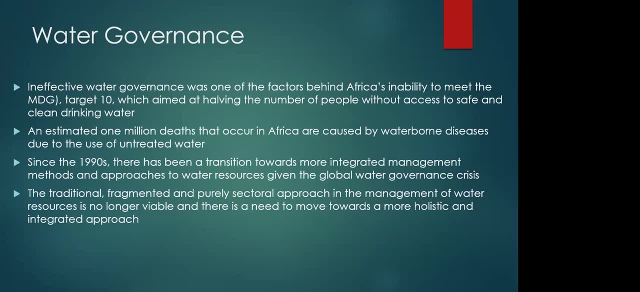 And we just wonder if we are going to meet SDG six. You see we are still talking about more than a million depth- that okay- in Africa caused by waterborne diseases due to the use of untreated water. So since the 90s there has been a transition. 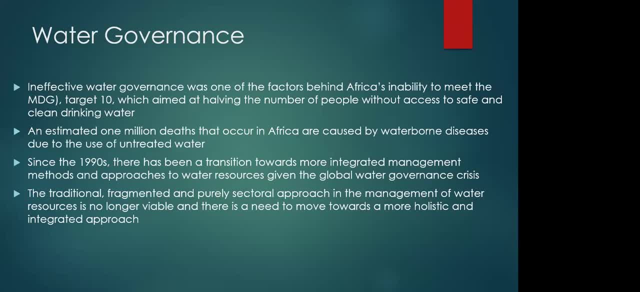 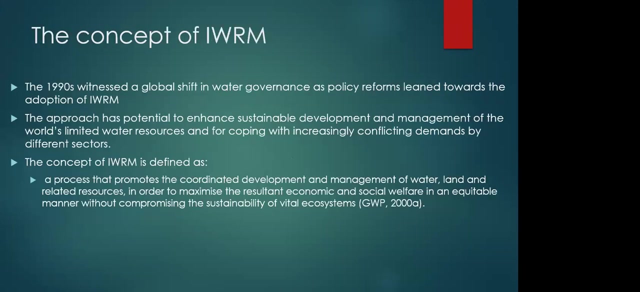 towards more integrated management methods and approaches to water resources. given the global water governance crisis, The traditional fragmented and purely sectoral approach in the management of water resources is no longer viable and there is need to move towards a more holistic and integrated approach. So the 1990s witnessed a global shift in water governance. 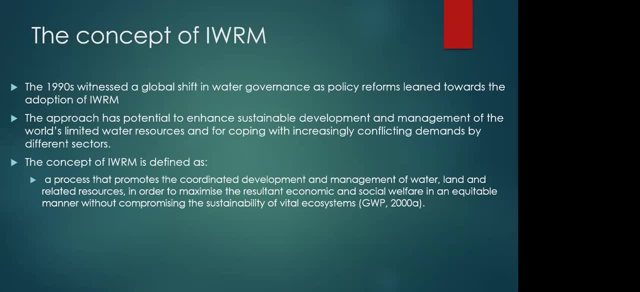 as the policy reforms leaned towards the adoption of IWRM. So the issue about IWRM, it's something developed at the global level, but now we have to. if we adopt it, we have to domesticate it. It has to fit in our contexts. 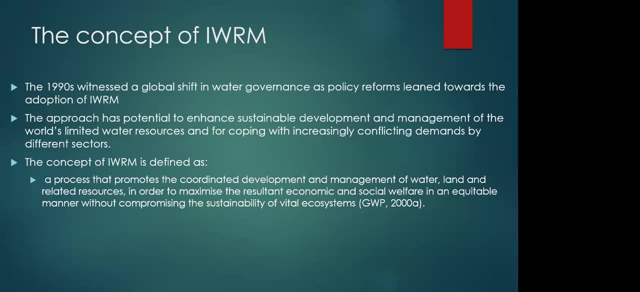 like what we are talking about. It has to take into consideration our societies, It has to take into consideration our cultures. So we just don't have to adopt it as it is. You see, we have to make it relevant, make it appropriate. 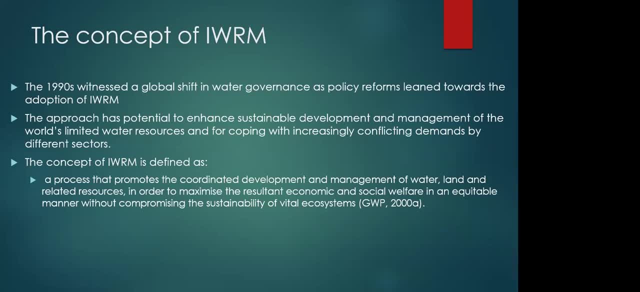 but what that means, its basic or its core principles? they are present. So the approach has the potential to enhance sustainable development and management of the world's limited water resources and for coping with increasingly conflicting demands by different sectors. So the concept of IWRM is defined as a process that promotes the coordinated development. 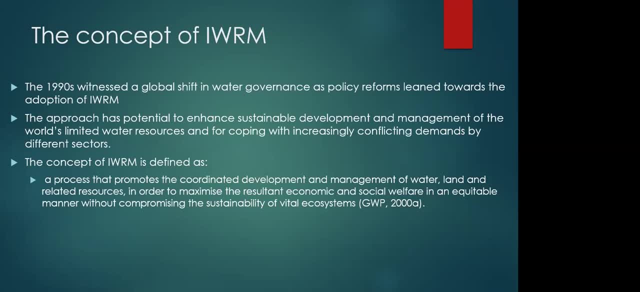 and management of water, land and related resources in order to maximize the result of economic and social welfare in an equitable manner, without compromising the sustainability of vital ecosystems. I'm sure you dealt with this, Moria. could you please mute those with unmuted mics. 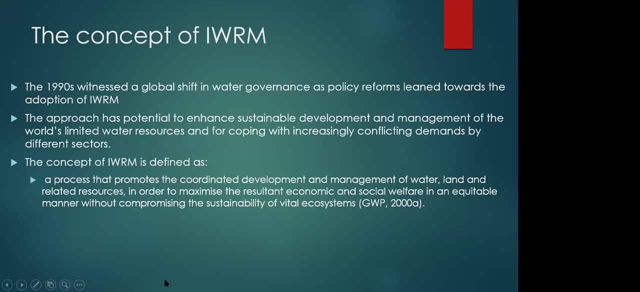 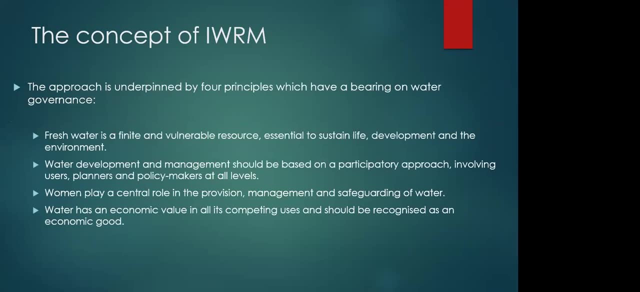 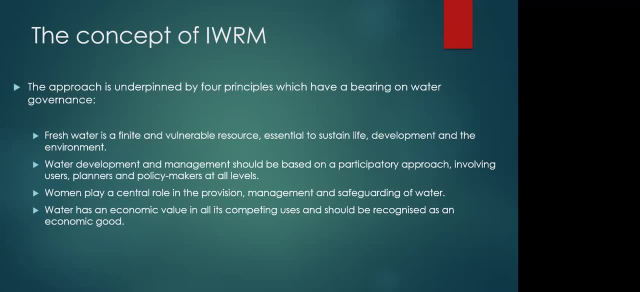 maintenance. So the first principle: we are saying: fresh water is finite and vulnerable resource essential to sustain life, development and the environment. So once you say fresh water is finite and vulnerable, that forces you to put into place rules, regulations, institutions. 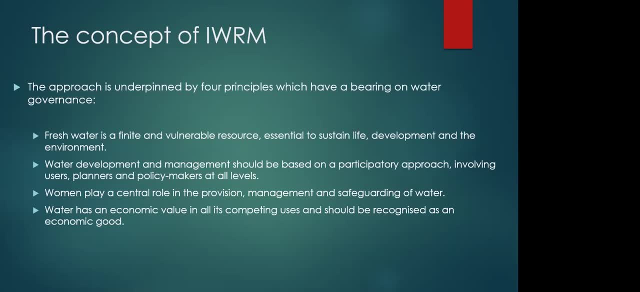 and policies, You see, in the hands of its sustainability, You see, so that it sustains life, so that development, you see, is not hindered. And then the other thing is that water development and management should be based on a participatory. 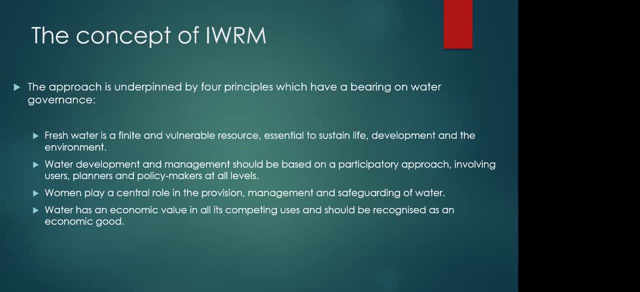 approach involving users, planners and policymakers at all levels. No one should be left behind when it comes to the issue of water resources management. When you say users, now link that to the culture that we are talking about, Link that to the society that we are talking about. 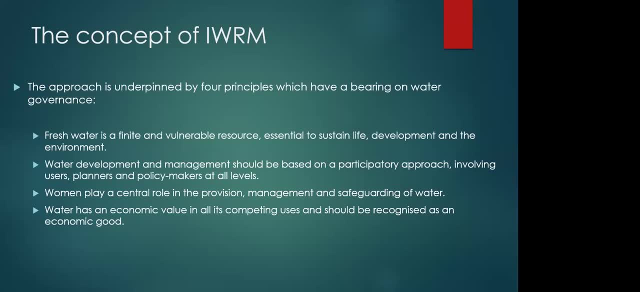 Users belong to a particular society. Users have a culture, So IWRM now takes into consideration their culture, their society, their customs taken into consideration, And then the planners, and then the policymakers at all levels, And then the other thing is, women play a central. 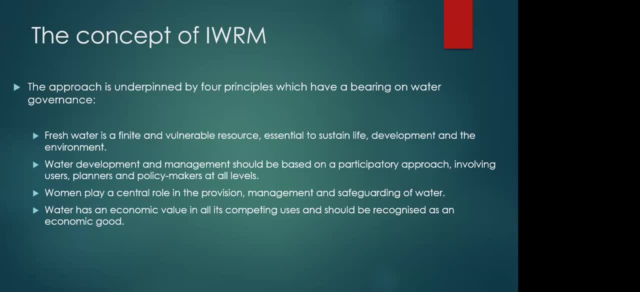 role in the provision, management and safeguarding of water resources. You see, so this was actually put in place, particularly taking into consideration of Africa, Asia, where women are central in the provision of water resources. They should not be, you know. 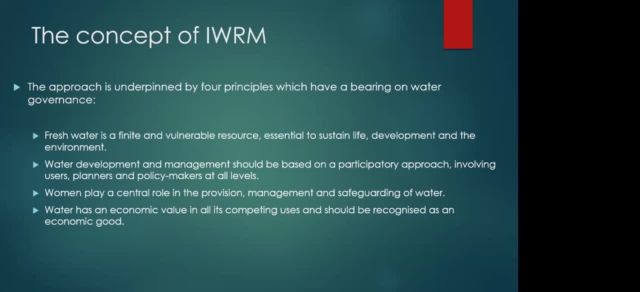 they should not be left behind. So the last principle is that water is an economic value in all its competing uses and should be recognized as an economic food. Yes, we know that no one should be denied water, But water resources when they are developed. 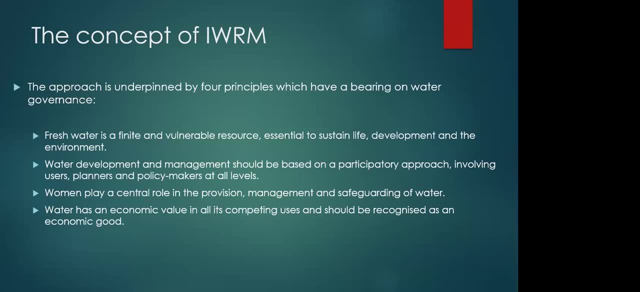 you see, when you damn the water resources, when you have to provide water resources of a certain quality, when you have to convey the water resources for either domestic or productive purposes, there is a cost. You see, there is a cost. from where? it starts from, There is a cost. You see there is a cost. from where it starts from, There is a cost. You see there is a cost. You see there is a cost. You see there is a cost from where it starts from. 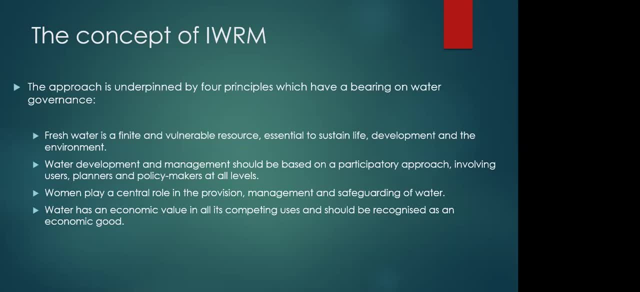 To the consumer. there is a cost, And who should pay that cost? The user has to play his or her part in meeting that cost. Our government has to play their part in meeting that cost. So the cost might be very expensive to the end user. 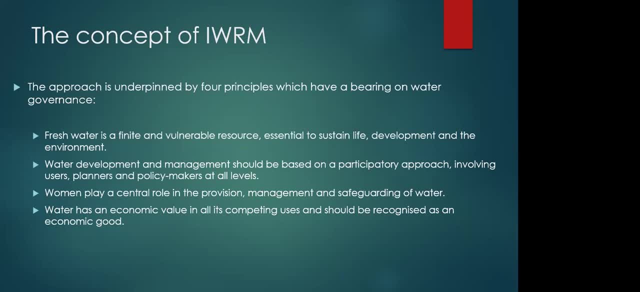 We know that poverty is rife in Africa. Some users, some users might not be able to pay, And then that's where government subsidies come into place. Maybe the government will say: you pay a certain percentage and then the other percentages to be paid. 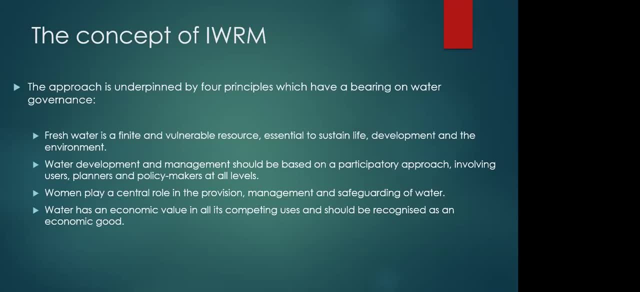 by the government, You see, And then that should go to the water supplier. not just that. the user pays maybe 50% of the cost And no one is meeting the other 85% of the costs. The water supply system will just collapse. 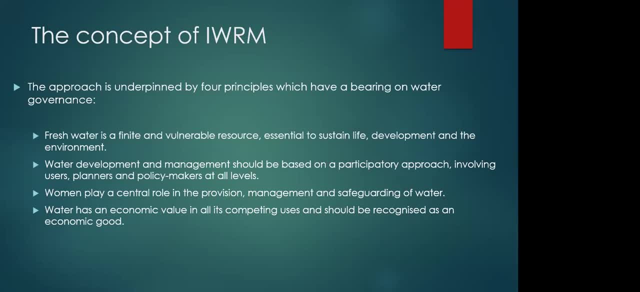 You see. So let's take into consideration this economic component, But let's balance it with the social part. Any questions or any comments? If no one has so-called companies, this is the Marshall Plan. There are also several other organizations who are. 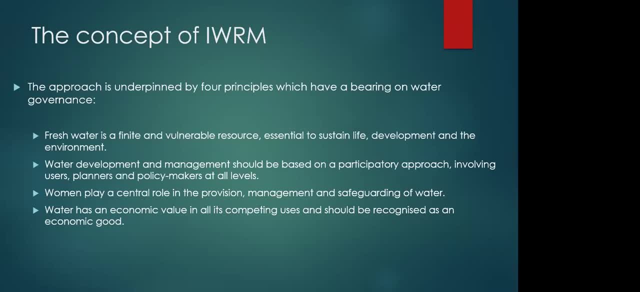 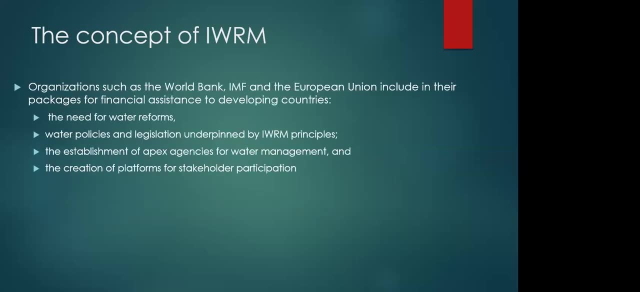 able to implement a lot of those policies Based on the principles of IWRM. So all these things have to be underpinned by policy, They have to be underpinned by legislation, And then you have institutions, you see, which make all these principles happen. 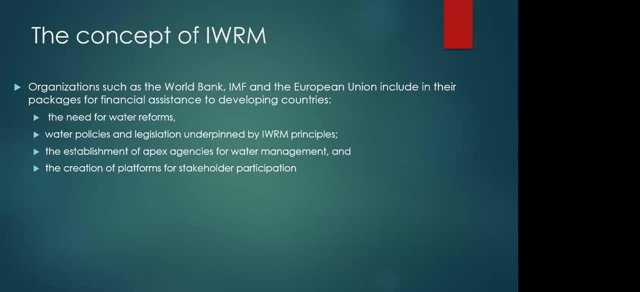 So organizations such as the World Bank, IMF and the European Union. they have a need to create a trend, And if it's not an idea, they shouldn't be doing it- and the European Union include in their packages for financial assistance to developing countries. 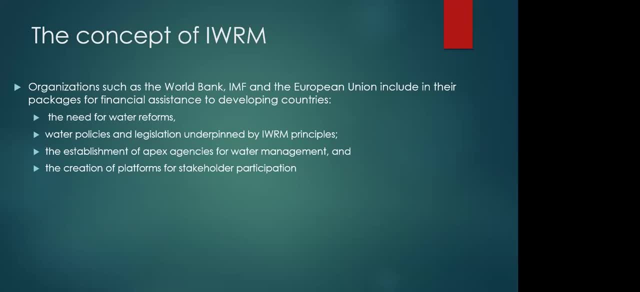 the need for water reforms, you see, And in particular, IWRM-oriented water reforms. You'll find that countries like Zimbabwe, Tanzania, Australia- we all implemented our water reforms during the 90s, When we were having these packages, financial packages. 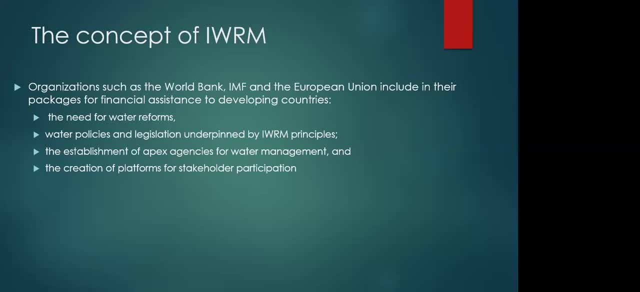 from the World Bank and the IMF. So hello, Yes. so you said any reactions there before I wanted to make a reaction on the principles of IWRM. Okay, In particular principle number three, which talks about the importance of women. 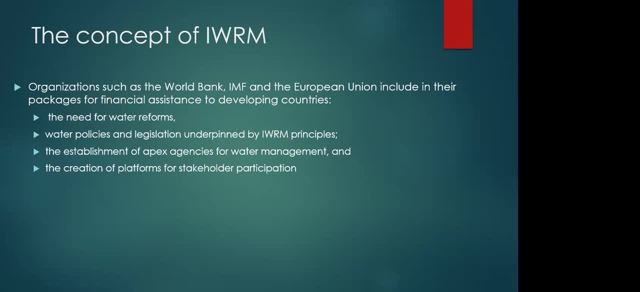 And you. you also mentioned that it was mainly for Africa and Asia, where our system of socialization makes women kind of more important in water. But do you think this principle is still worth it, or maybe things have moved on and we might need to also have a rethink about this principle? 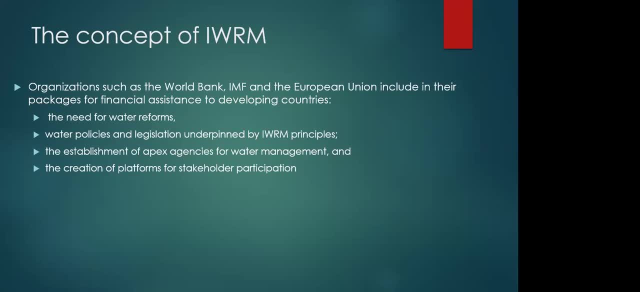 Okay, thank you. Any reactions before I come in? Yes, Bina, do you want to respond to Thessie here? Anyone who wants to respond to him? Okay, I personally think that the principle is still valid. Look our population. 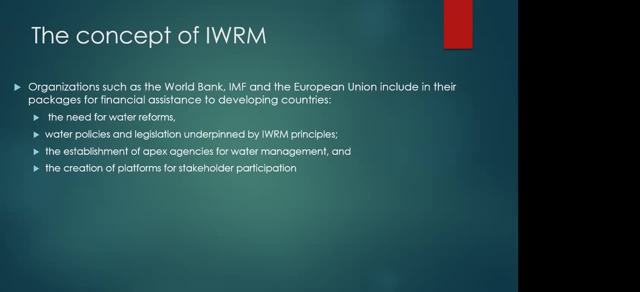 the majority of our population is still rural, Even in the urban areas. I will tell you why. I also say in the urban areas. it's also valid. Women are responsible for ensuring that there is water at the household level. They still have to travel. 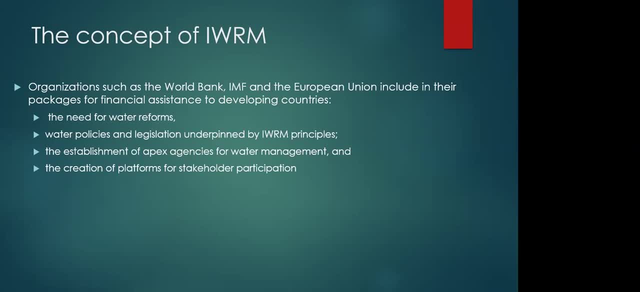 Okay, I'll give you an opportunity. They still have to travel some distance to go to a water source And if you look at most of the publications, you see that water sources for domestic purposes, they are frequented by women, They are managed. 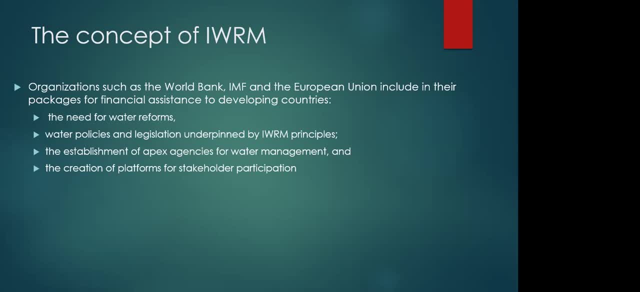 by women. But where there is a difference is on productive water. When it comes to productive water, men dominate, you see, because we are talking of something that is commercial now, you see, So that also still is valid, because you want. 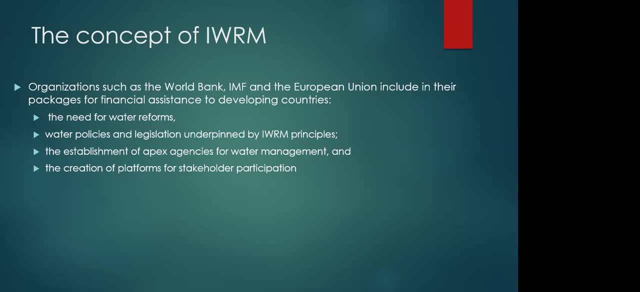 women to also access domestic water. I mean productive water. You want women, you see, not to walk longer distance to access domestic water. you see Water, they should access water within reasonable distance. They don't have to walk very long distance. They don't have to spend all those you know hours. 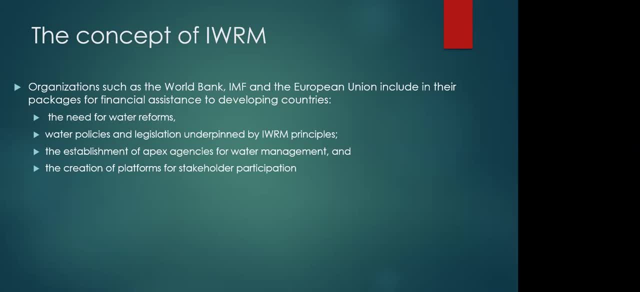 Women spend, you know, per year. you see, in some of the raw areas You are talking of, you know maybe 500 hours. you see a woman has to spend, you know, maybe going to a water point and then coming back, And also they have other duties to perform With school-going-age girls. 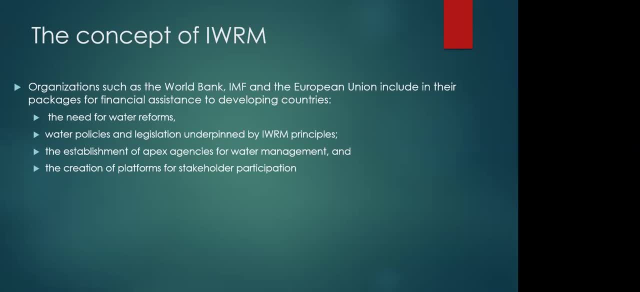 it's the same. Maybe in the morning they have to go and fetch water. After that they have to go to school. After school they have to, you know-and then-and the cycle continues, you see. So, given that fact –. 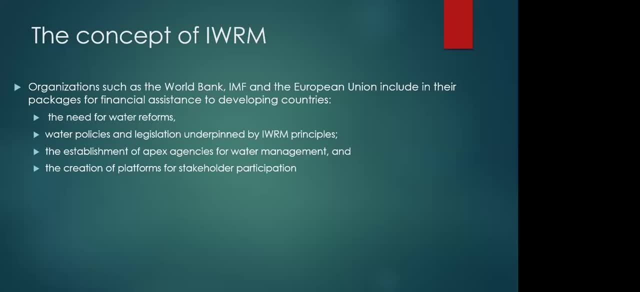 Why? Why not involve them – kindly mute your mics, please, Please-why not involve them in the management of water resources? they should be there in every in all the structures which are responsible for water resources management. you wanted to comment on something. 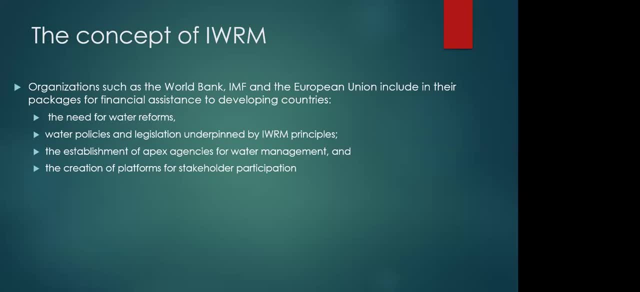 can you? yes, just my thinking that in this 21st century- and I realize what you have said and I also agree that it's quite important- but doesn't it propel kind of the marginalization of women or kind of I mean, why should they be streamlined? 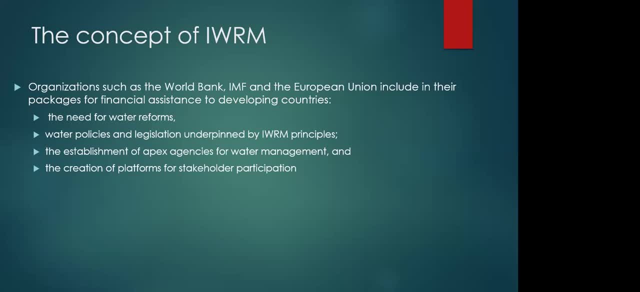 in that case, I think we should. men and women are. you think it's very important? but you're talking about this one. that was my take. maybe we can take it okay from a gender perspective, because when we are talking about gender, we are talking about men and women. 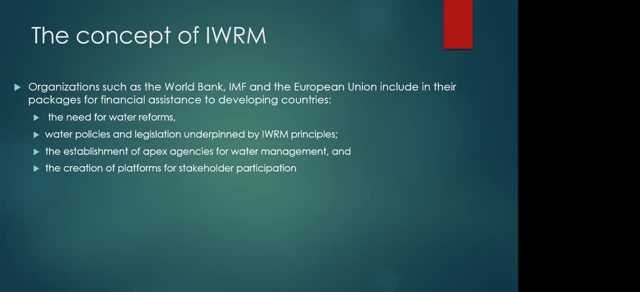 you see? so from a gender perspective, we are saying we don't have to lose sight of the fact that women have been disadvantaged and they are still disadvantaged. let's not be gender blind and pretend as if women are not disadvantaged at the moment. they are still disadvantaged. 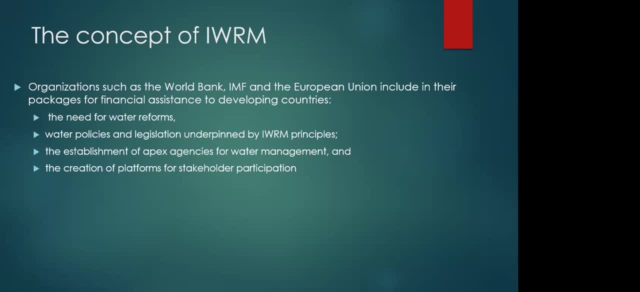 so it's important for them to be involved, or for them to be singled out, you see, so that they take part in structures that are responsible for water management. I don't know what others think. of course, this is a debatable. it's a debatable issue. 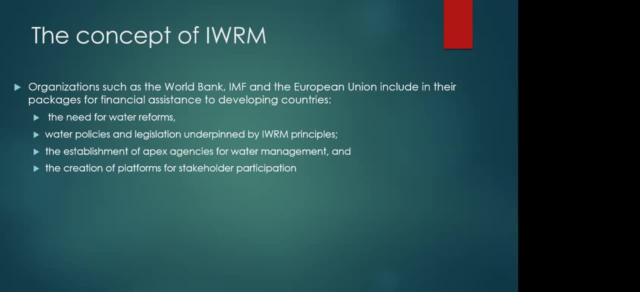 you see, I agree where you are coming from, but it's debatable. it depends on where you are standing. okay, anyone who wants to. who wants to comment on that as well? okay, Moses is saying: women have significant specialized IKS knowledge that is relevant for IWRM. 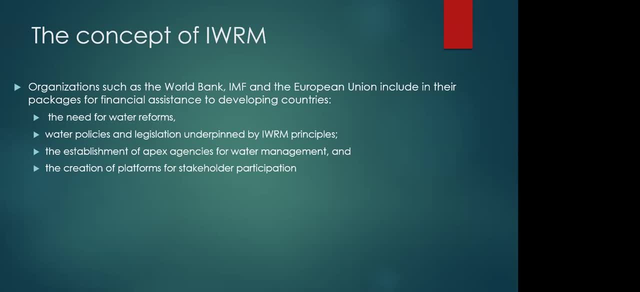 I don't know, Moses, if you want to elaborate, maybe you can unmute and elaborate on that. okay, I don't know, Moses, if you want to elaborate, maybe you can unmute and elaborate on that below. yes, because they are, because they are for the showed, because they are. 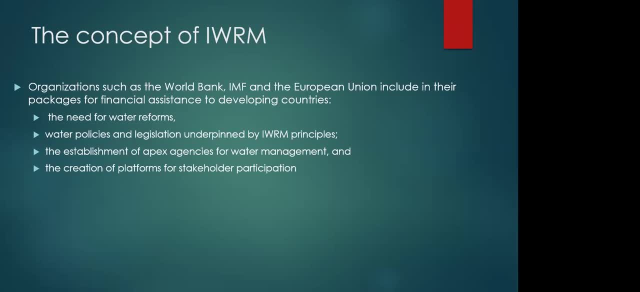 responsible for the supply of water for the domestic and primary use, for the home. so because of that they are experienced in the supply, so they tend to possess that specialized knowledge which is very important for the integrated water source management. Yeah, but I think his person, his argument, 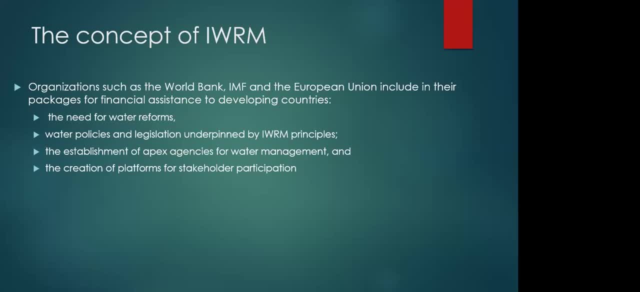 is why should we talk about this? He is talking about other things, but I think this is important. or is he talking about what young girls do, asking you: take a lot of images into their mind. perpetuate that, you see. should we? should we perpetuate that? can't that be shared? 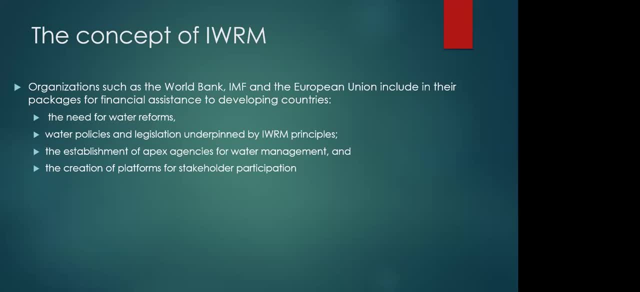 you should understand that the society has got roles. we don't have to deny that. so if it's important, we need to be specific when we are planning, when we are planning this integrated water resource management, such that we know that everyone has got this role we don't have. 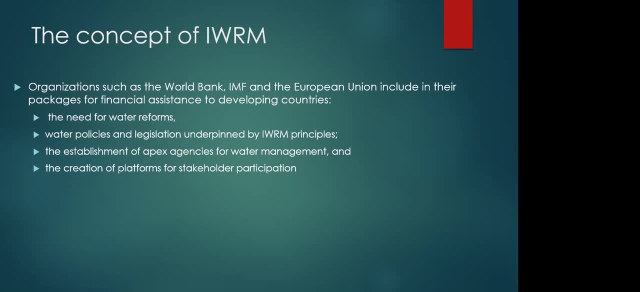 to deny things that are there. we know that in the society, especially the african society, women and men, they've got their own roles. so it's very important when you are planning for an integrated management, so that we consider these roles in our framework. i don't know whether you get it okay. 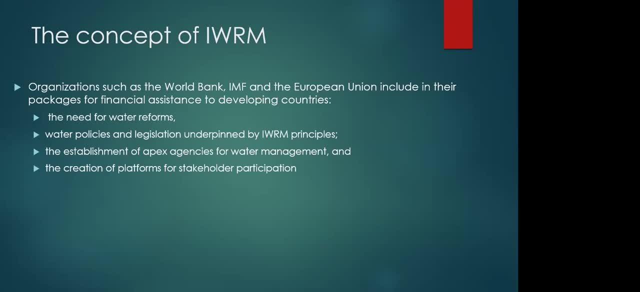 okay, that's uh, that's okay. thank you, uh, very debatable indeed. okay, let's uh, we need to move first now. uh, i thought by now we, we should have been done. uh, thank you for those interventions. uh, i'm sure we had gone through what's on the 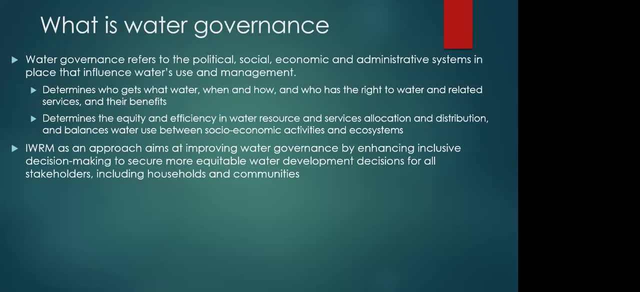 uh, on the screen. so what is water governance that we are talking about? so what a governance refers to the political, social, economic and administrative systems in place that influence water use and management. so it determines who gets, who gets what water, when and how, and who has the right to water and related services and their benefits. it also 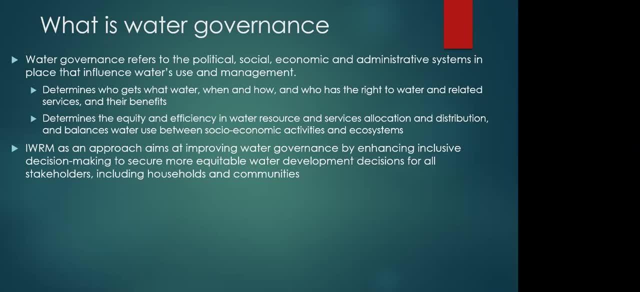 determines the equity and efficiency in water resources and services allocation and distribution and balances what are used between socio-economic activities and ecosystems. so iwrm, as an approach, aims at improving water governance by enhancing inclusive decision making to secure more equitable water development decisions for all stakeholders, including households and community. so water governance is something which is very uh, which is. 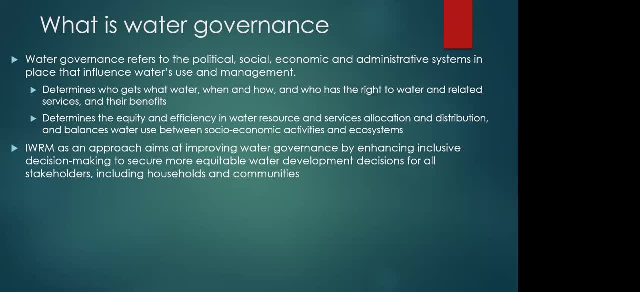 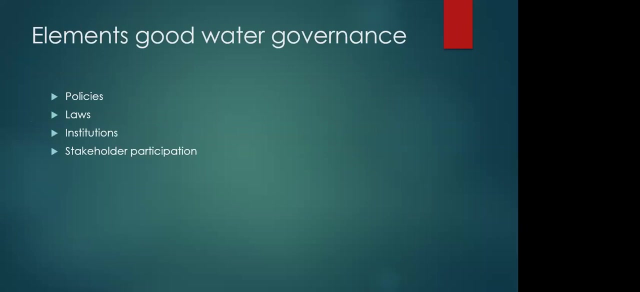 very broad and all its different systems. now they have to be, they have to be balanced if you are really going to ensure sustainable water use and management. so what are the elements of good water governance? we are talking of policies, we are talking of laws, we are talking of institutions. we are starting with stakeholder participation, but in the stakeholder. 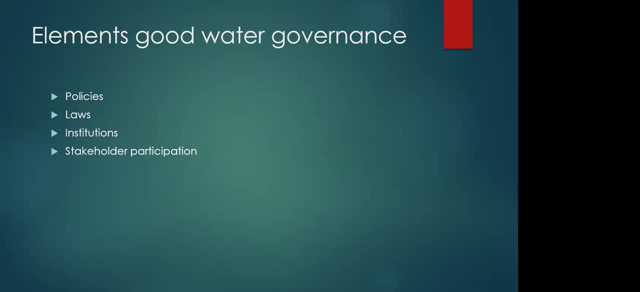 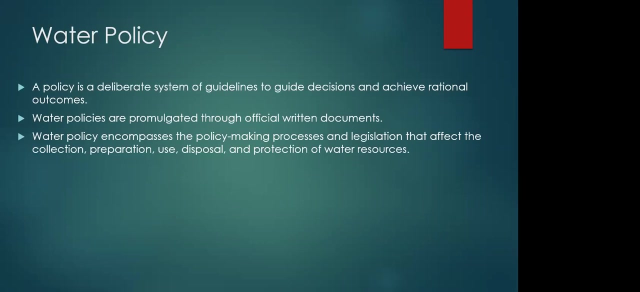 participation comes under institutions and also is underpinned by those policies and laws. so the first three: they are the most important or they are the key elements of of water governance. so when we are talking about a water policy, we are talking about a deliberate system of guidelines to guide. 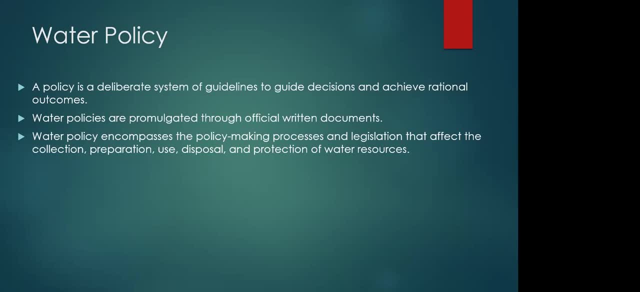 decisions and achieve rationality outcomes. So water policies are promulgated through official written documents And they encompasses the policymaking process, legislation that affects the collection, preparation, use, disposal and protection of water resources. So you basically need to understand. there's a 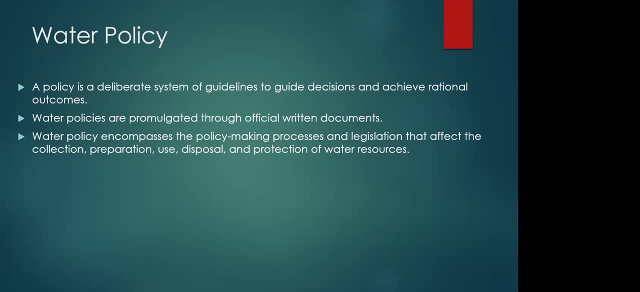 difference between a policy and a law. you see A law, you enforce it. you see It's a rule, you see. But policy, you see, it's something which is an official standard of a ministry, of a government. It's a guideline And usually 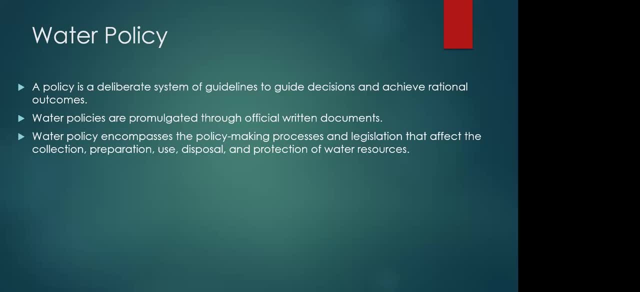 I'm not a lawyer, but you cannot really argue in courts on the basis of a policy you see. So when you want to make it a rule, to make it more enforceable, you then put a law you see, So it's debatable at times. 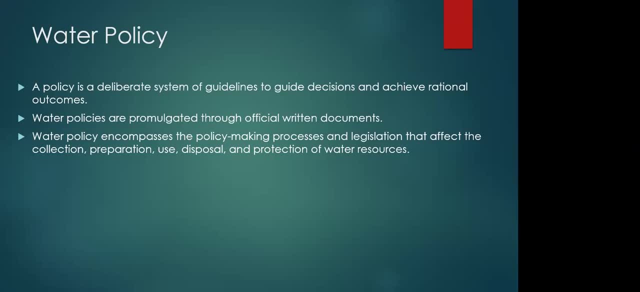 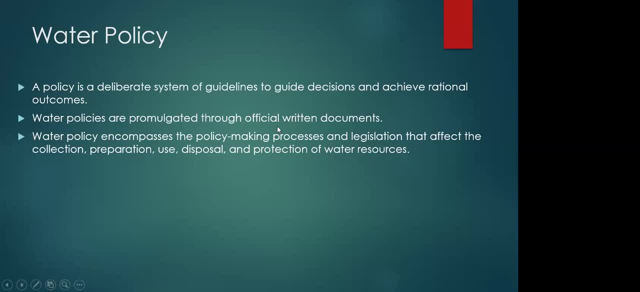 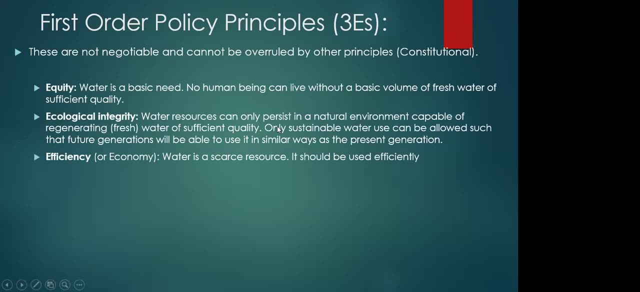 Any lawyer, Any lawyer, Any lawyer, Okay. And then, when you are talking of law, I mean policies, Policies as principles, you see. So you have what are called first order policy principles, like in water, they are the three E's, you see, which are the first order principles, which are very important. 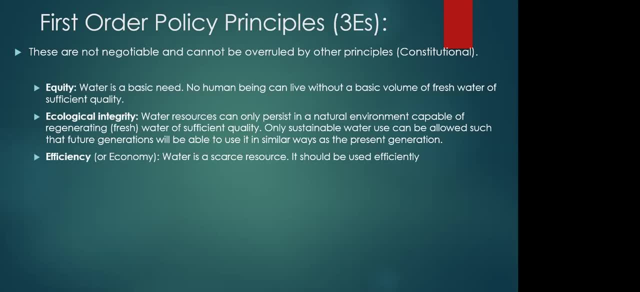 and even globally, they are accepted. you see, We talk about the issue of equity issue of water is a basic need. No human being can live, not only human beings, animals, plants can live without a Okay Of fresh water. you see, of sufficient quality. You talk of ecological integrity, Water resources. 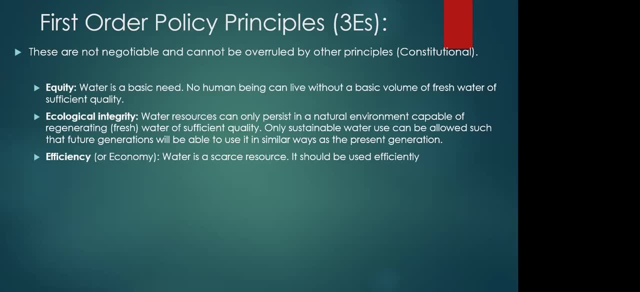 can only persist in the natural environment of capable of regenerating fresh water of sufficient quality. Okay, great, Thank you, Dr Kujinda. Dr Kujinda, you have your microphone. Hello, Dr Kujinda, Dr Kujinda. 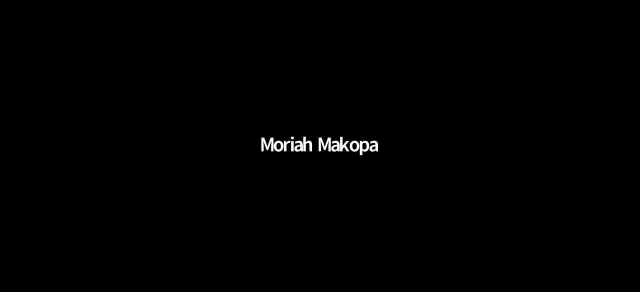 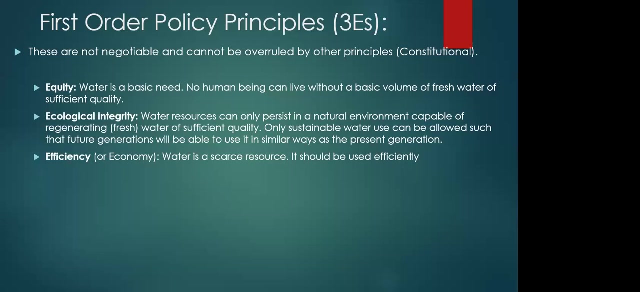 Sorry, Sorry, I've been kicked out again. You're welcome. You're welcome, I'm sorry, Sorry, I had to get out. I'm sorry, I was really really sorry. Any other questions again? okay, yeah, okay, so maybe we have to, we have to just uh rush. so i was talking about those three. 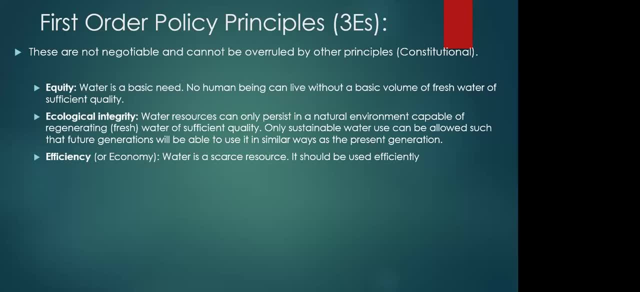 is i'm sure you you followed me on uh on the three is you see the first order policy principles: equity, ecological integrity and efficiency. if you go in any uh global uh documents you earn, or any other uh uh organization or our regional sada can suffer. they emphasize on these principles. 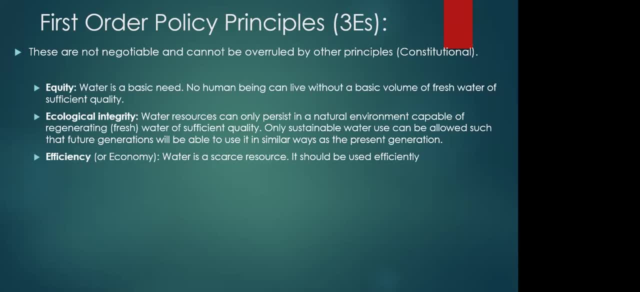 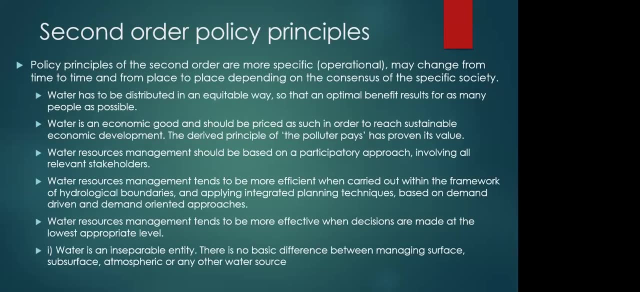 even iwrm also emphasize on these principles. and then they are what are called second order policy principles. these are policy principles of the second order which are more specific, operational. now they may change from time to time and from place to place, depending on the consensus of the specific 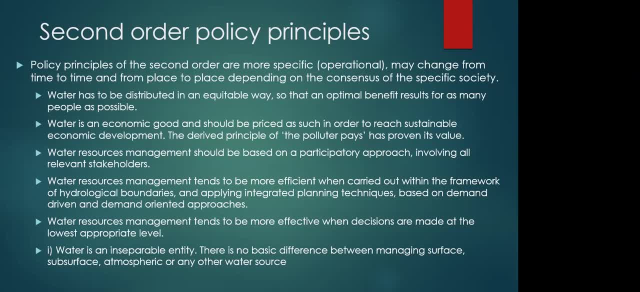 society or nation. you see, water has to be distributed in an equitable way so that optimal benefit results uh for as many people as possible. water is an economic good. it should be priced as such in order to reach sustainable economic development. uh, water resources management should be based on a participatory approach. 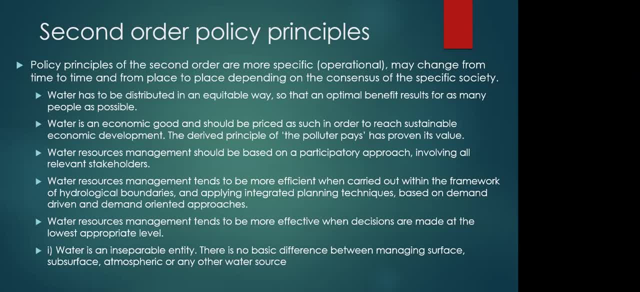 involving all stakeholders. water resources management tends to be more efficient when carried out within the framework of hydrological boundaries and applying integrated planning techniques based on demand driven and demand oriented approach. water resources management tends to be more effective when decisions are made at the lowest appropriate level. 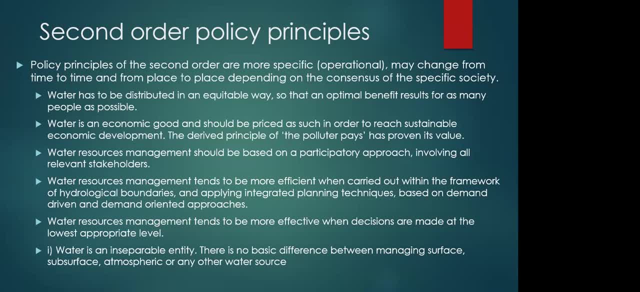 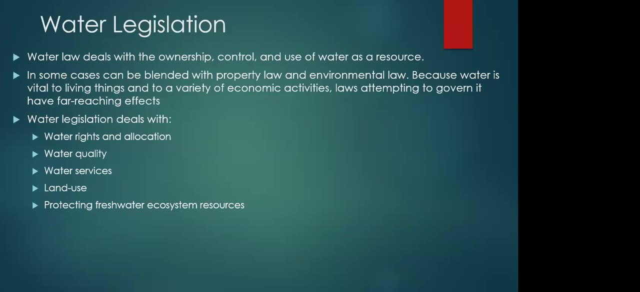 water is is an inseparable entity. there is no basic difference between managing surface, a surface, subsurface, atmospheric or any other water source. so those are second uh order principles. and then, when we come to what is legislation now, we are now dealing with uh, with laws, you know which? 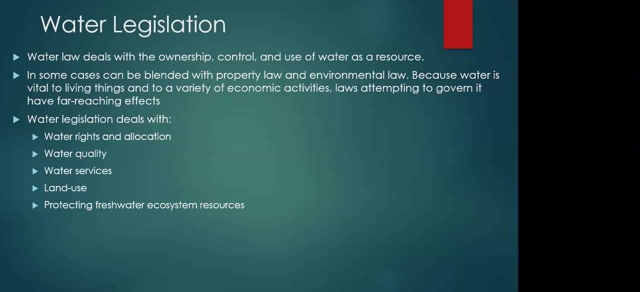 talk about ownership, control and use of water resources. in some cases it can be blended with property law or environmental law, because water is vital to living things and to a variety of economic activities. so laws are attempted to happen: eating far-reaching, equal- yeah, i mean effects. so what are legislation it deals broadly with? 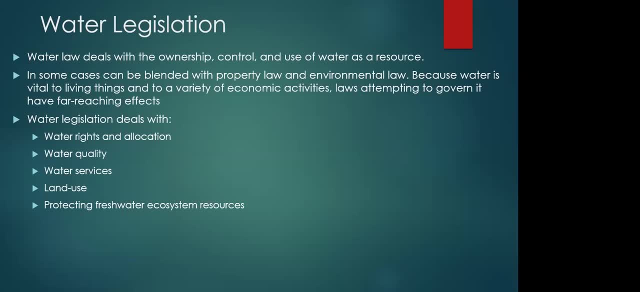 the water rights and allocation. water quality: what is the quality of water? water should be of a certain quality. what are services? who provides the service? in your country? there is a particular organization which provides the service In Zimbabwe. we are talking at the national level. we are talking of the Zimbabwe National Water Authority. 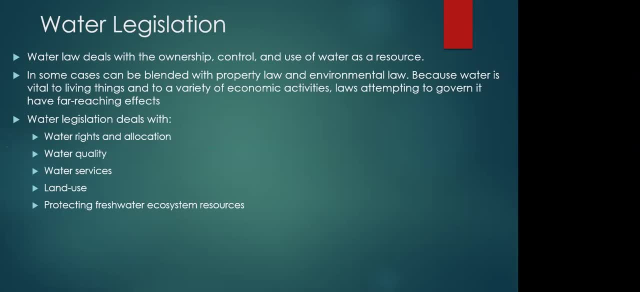 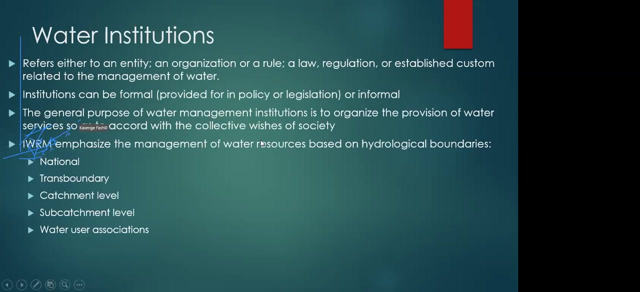 In South Africa. maybe you are talking of the Department of Water Resources, DWA. It also deals about the issue of land use. It deals about the issue of protecting freshwater ecosystems. So those are some of the issues which water legislation deals with. 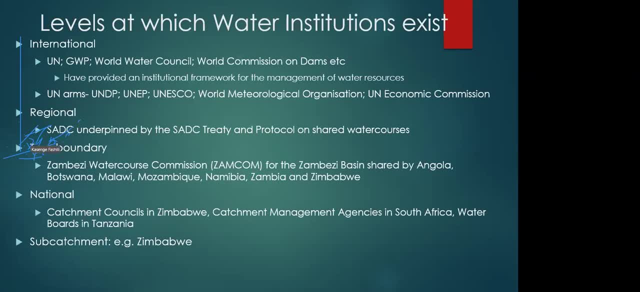 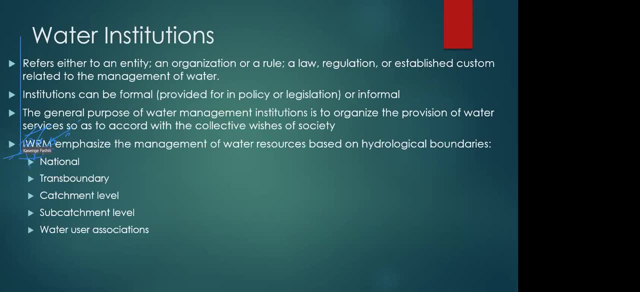 And then, what are institutions? What are institutions? So these refer to an entity or an organization or a rule or a law, a regulation or established customs related to the management of water. So institutions can be formal provided for in the policy or legislation. 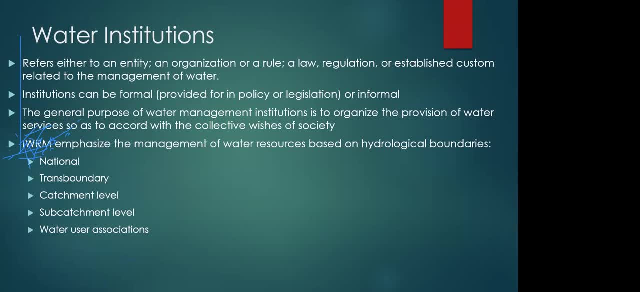 Or they can be formal. So the general purpose of water management institutions is to organize the provision of water services so as to accord it with collective wishes of society. So this IWRM basically emphasizes management of water on hydrological boundaries. It can be within a country at transboundary level. 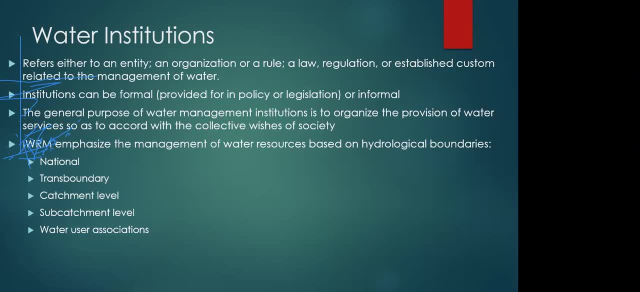 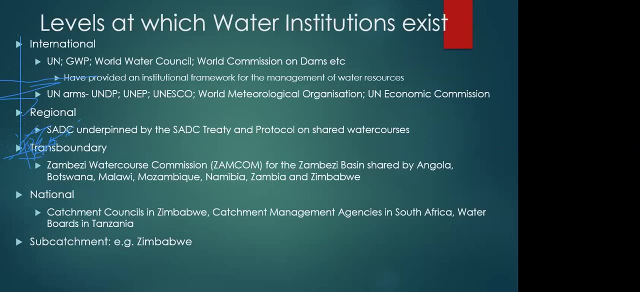 at catchment level, at sub-catchment level and at water usage. You see. and water institutions, they exist at different levels. We have these at international level, like your UN, Global Water Partnership, World Water Council, World Commission on DEMs, you see. 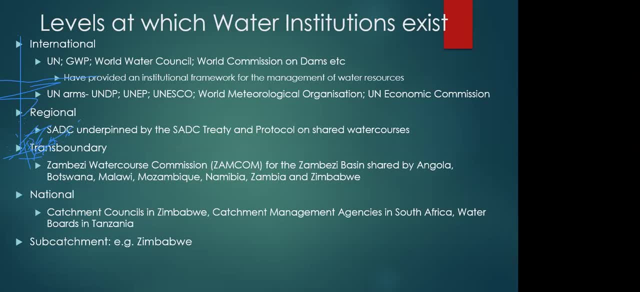 And you have also other UN arms At the regional level, for example in Sudan. we have the, And then you have the World Council on Water, the World SADC- Southern African Development Community, underpinned by the SADC treaty and a protocol. 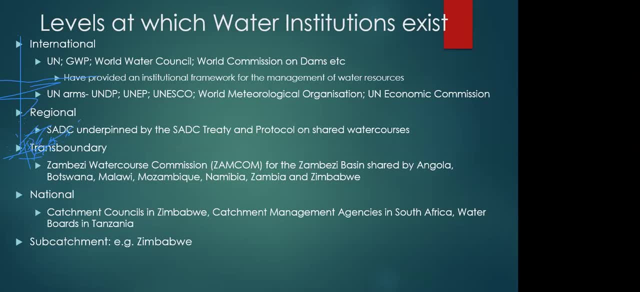 on shared waters, And that protocol, you know, gives room for the creation of our basin commissions, like the Zambezi Water Coast Commission, which is shared by seven countries. We don't only, it's not only- Zamcom. we have Orasecom for the Orange Senku, we have 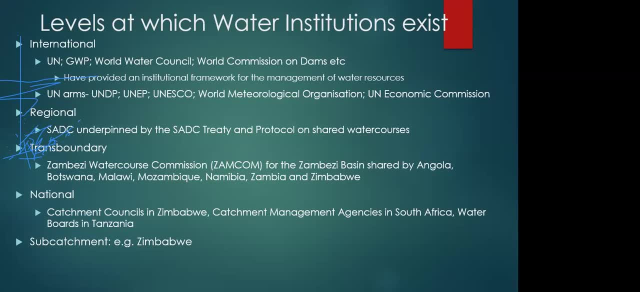 Limcom for the Limpopo, we have Kunene, you know, for all the 15 river basins that we have, And we have national at national. we have catchment councils in Zimbabwe, catchment management agencies in South Africa, water boards in Tanzania. 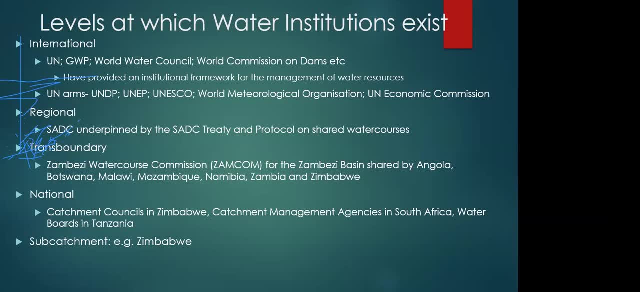 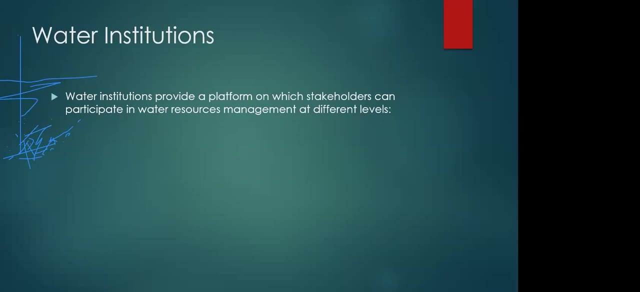 And then we have sub-catchments. for example, in Zimbabwe and other countries they have sort of similar institutions, So water institutions. now they provide a platform on which stakeholders can participate in water resources management at these different levels: at national, at regional, at transboundary. 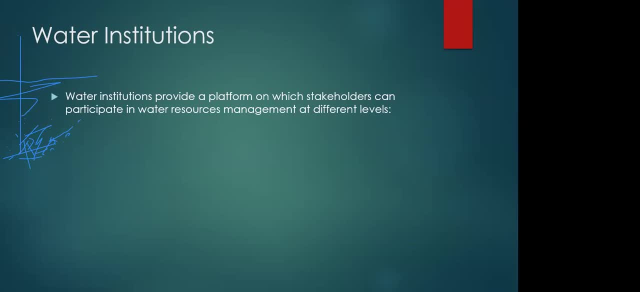 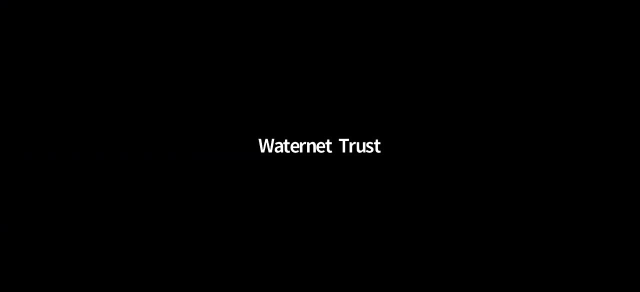 at sub-catchment and catchment levels. I'm sure I am done now Any questions? Any questions Or comments? Am I still in the meeting? Yes, Yes, you are Okay. Okay, Thank you. Can we have questions? 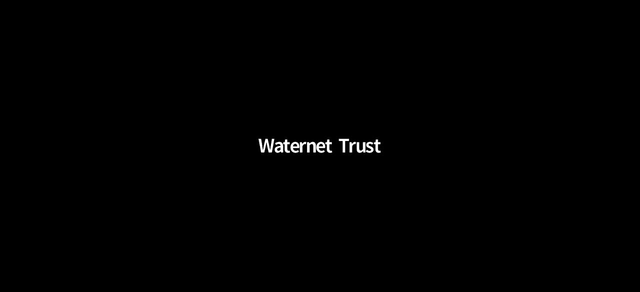 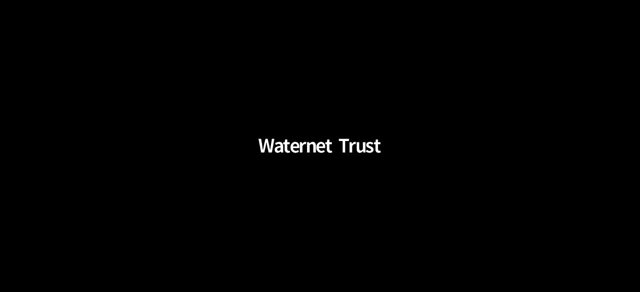 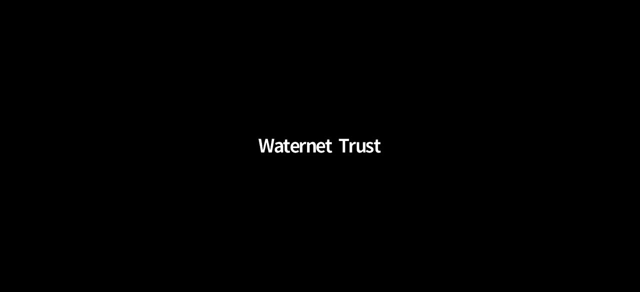 Yeah, maybe, maybe you can post it. Maybe we can have some comments on water governance structures from your countries. What are your experiences? You have said No. Why is this a question? What are the experiences from your countries in terms of water governance? 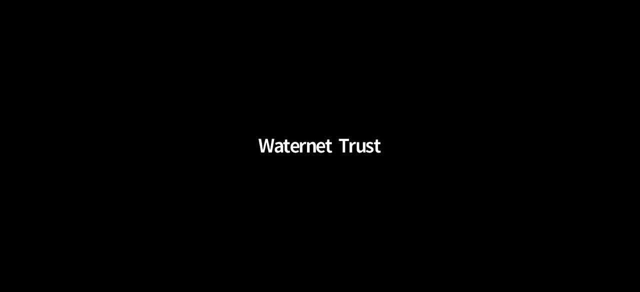 Are there any challenges? What are the challenges? What are the successes And which areas do you think our countries should make amends so as to improve water governance? Can you hear me- Yes, you can hear me- In terms of sitting water as an economic good. I think in our country institutions that 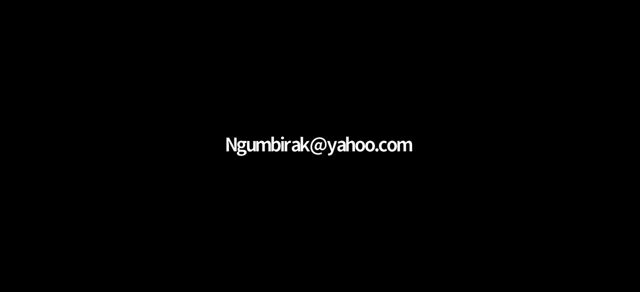 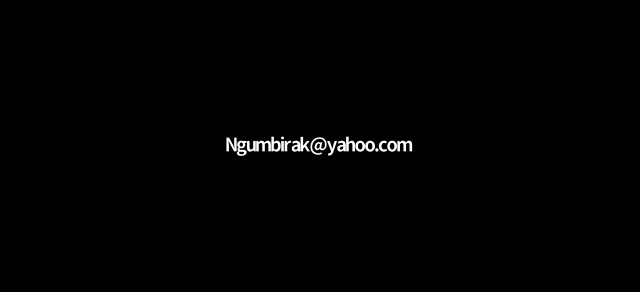 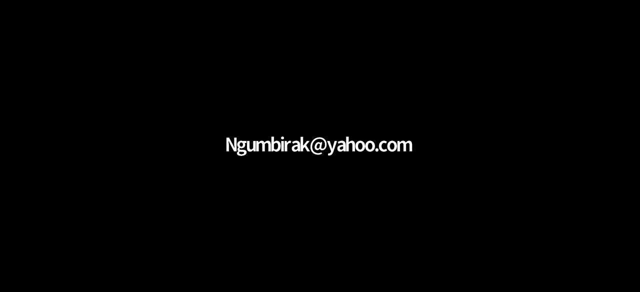 So they just raise the price of water any time. So maybe they can improve in those areas Could be much better. Okay, Okay, Thank you. Any other comments? Can we have some comments From other countries? Yes, Ngaba. 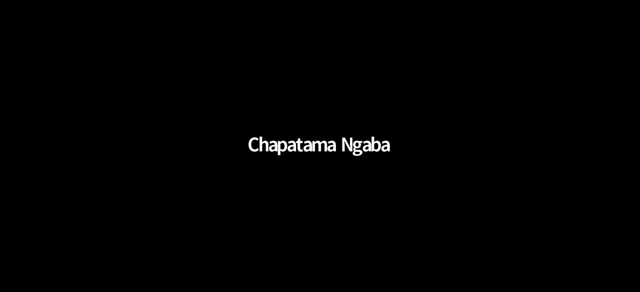 Yeah, so I'll speak from the Zambian point of view. What we have is the Water Resources Management Act. that provides for, first of all, WAMA, which is the Water Resources Management Authority. It also provides for the establishment of catchment councils, sub-catchment councils and water use associations. 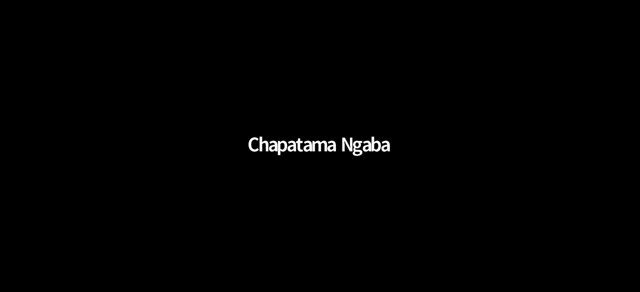 And obviously the aim of that is to decentralize the management of water all the way down to the water users themselves. But currently, due to lack of resources, the catchment councils, sub-catchment councils and water use associations have not yet been established. 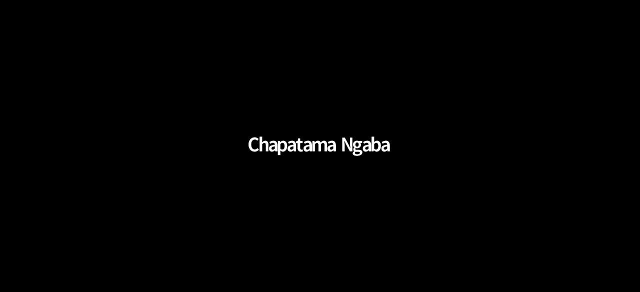 And what you have is just catchment offices in four of the six catchments in Zambia that assist in the regulating of the water resources throughout the country. So I think we need improvement in terms of having those structures fueled and resources provided for them to run effectively. 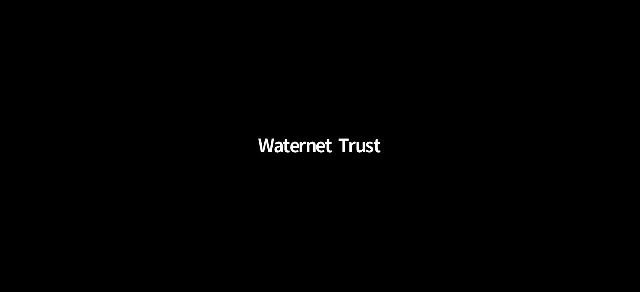 Thank you, OK, thank you, Very interesting indeed. As I have said, Zimbabwe also have catchment councils- seven catchment councils, you know, following the seven major rivers That we have in the country- And each catchment council is subdivided into sub-catchment councils. 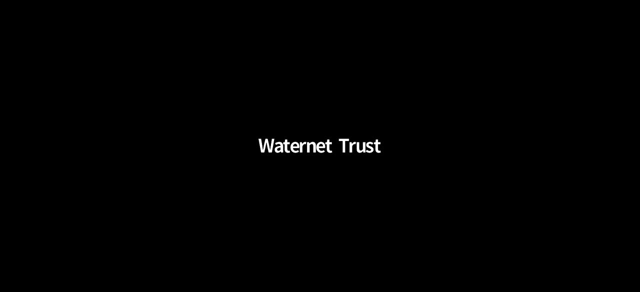 And below that we don't have any other structures. So it's interesting that Zambia has a structure below the sub-catchment council, The sub-catchment council that we have in Zimbabwe. you know, they are very big, you see, for management and operational purposes. 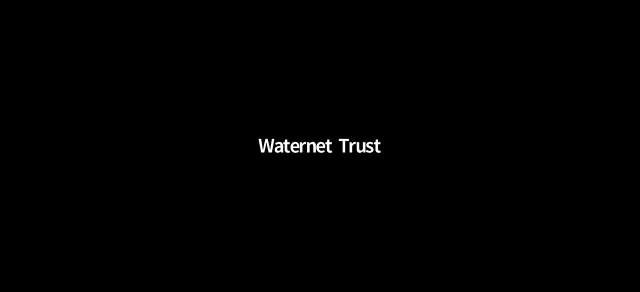 And one challenge that they are facing also is the issue of resources. just like what you are saying- Some of the sub-catchment councils- they cannot raise adequate resources for them to operate. Thank you. Any other comments? Do we have anyone from Tanzania? 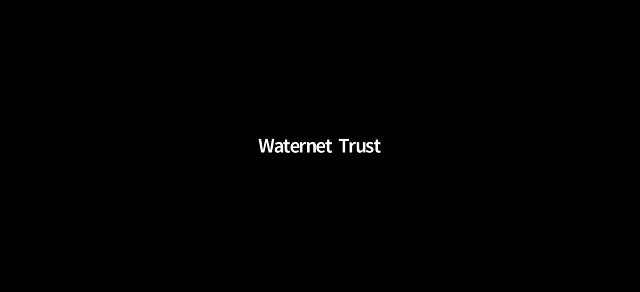 Tanzania, Lesotho, Swaziland- OK, Mamosa, Yes, Lesotho is one of the few countries that exports water, especially here in the Sadak region, But we have a challenge of development discourse: water scarcity in the lowlands. 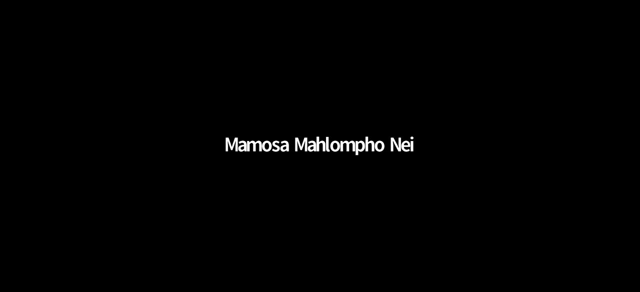 We export water, but the water within the communities of Lesotho is the problem, And we have discovered that the main problem for this is the infrastructure to manage this resource of water within the communities of Lesotho. That is all we have. 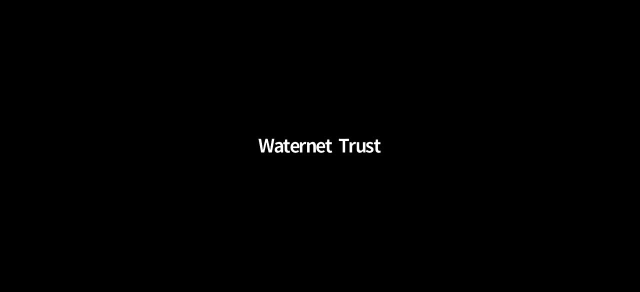 Yeah, very, very interesting indeed. You know, I'm not sure if there has been some studies to really look at what we are talking about. what has been the impact on Lesotho on exporting water? After exporting the water, does the country have in place a mechanism of saying, OK, they have earned so much and that much should be reinvested in the water sector? 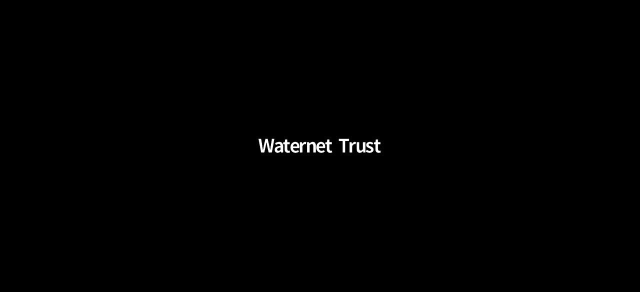 You see, to benefit the locals you know. So it will be interesting for those who are interested in studies of that nature, Or even a comparative analysis. As I was saying, Zambia has almost similar structures with Zimbabwe. What you know. how are these structures performing in these areas? 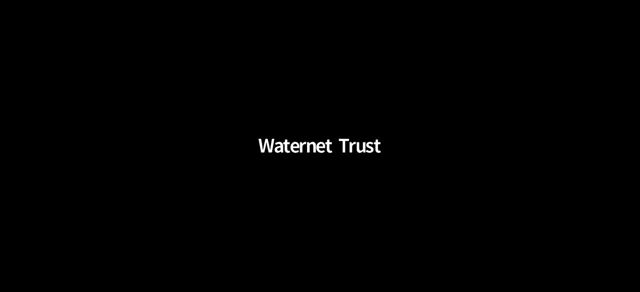 How are they performing in these countries? What challenges are they facing? So it will be very, very interesting for some of you to take up these studies. Any other comments? OK, let me check on the chat box. The challenge for Zambia in water governance is that governance issues are at a high level and not at low levels. 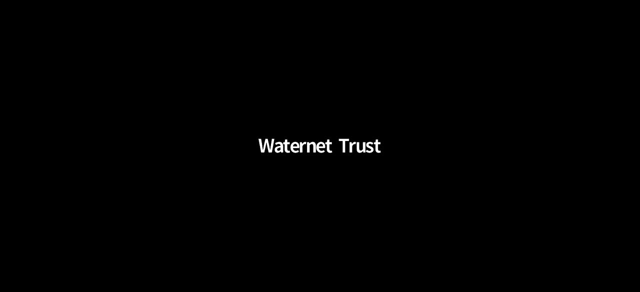 For example, small-scale farmers, who make the majority, don't know much about water governance. Cases of loom loom. same for catchment. Yeah, Even as I said, Zimbabwe has these catchment councils. They have been in existence since 2000.. 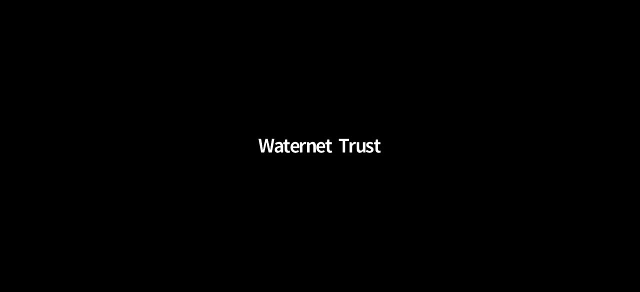 But you'll be surprised that some farmers or ordinary people within the catchments or the catchment councils don't know that they exist And they don't understand. you know how they, what their functions are, And then we have. is it a question or comment? 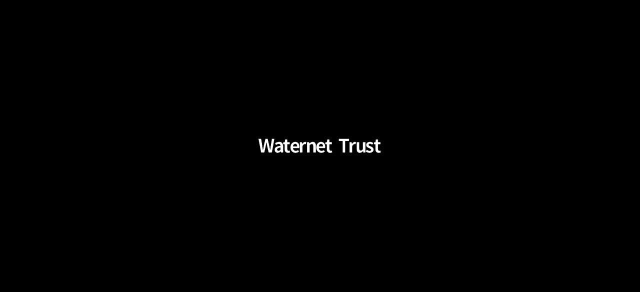 Does the World Council of Churches and other subsidiary faith entities have laid down any functional protocols for water governance? If not, why can't we learn from the mosaic ecological motif and God of Exodus, where Moses became the first hydrologist by striking a rock and providing water and went on to restore its quality, its mara? 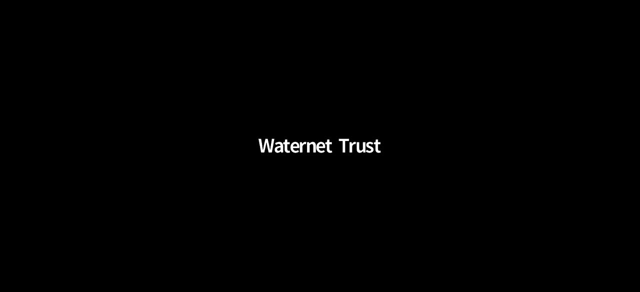 This should be our strongest motivation to develop faith-oriented protocols to provide governance and manage water resources. Yeah, very, very interesting. I'm not sure if these bodies have any protocols related to water resources management. It will be interesting for someone to look at this. 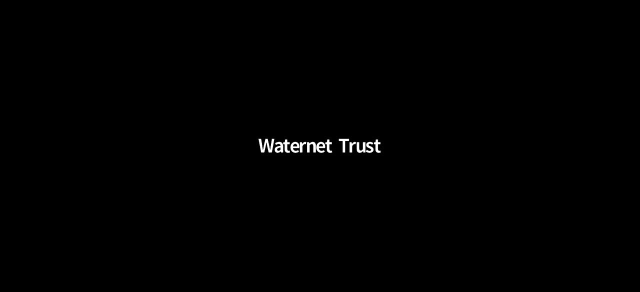 Okay, Any other comments? Mindu, would you like to say something? Sorry, I'm just trying to unmute my mic. There's a challenge, Okay, Okay, So if we don't have any other comments, Ladies and gentlemen, 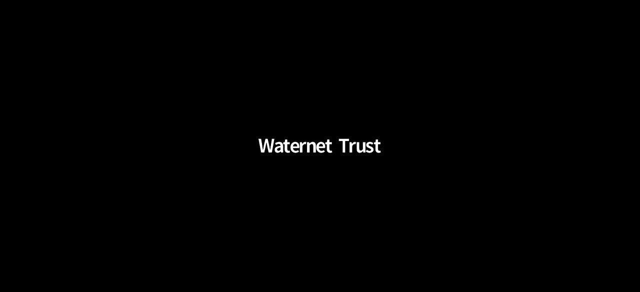 I would like to thank you for attending this live session. It's been very interesting. I've also learned, you know, new ideas from your comments. I will be posting a chat or maybe via email. Your assignment will just be one assignment. 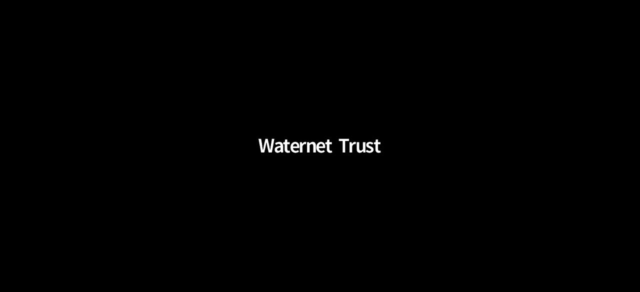 Not, you know not much. It will be very easy. So, thank you, I'm sure the next live session will be on Friday. We'll send you the link for the Friday live session, which will be in the afternoon, I'm sure between 3 and 4,, if I'm not mistaken. 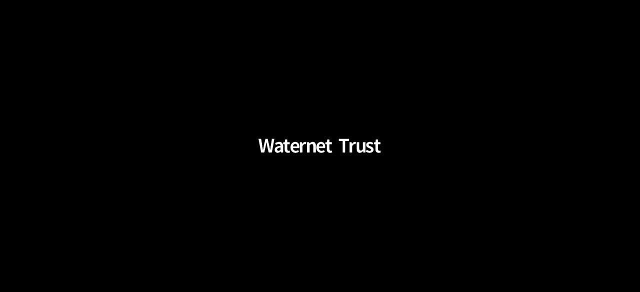 Okay. Okay, So we'll put the presentations on the platform, Unless if there is someone who wants to say anything. we have come to the end of our live session. Maybe, before we go, can we put our own videos and maybe have a photo. 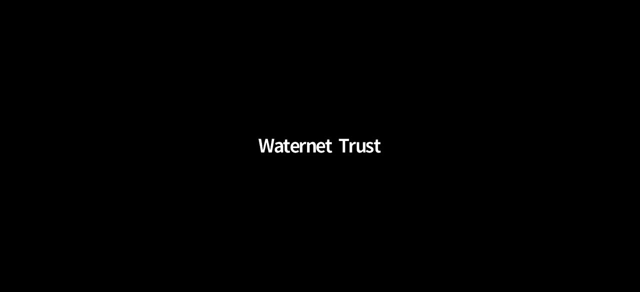 I don't know how to have all the. Anyone who knows how to have all the participants on the screen? I don't. I'm still seeing participants on top there. how can we have them on the screen? anyone who knows how to do that? okay, you go up there. hello, hello, yes, yes, there is on your, on your right. 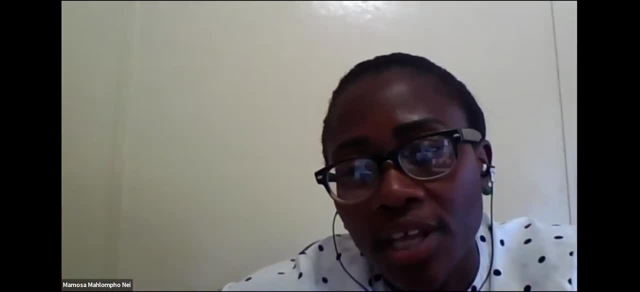 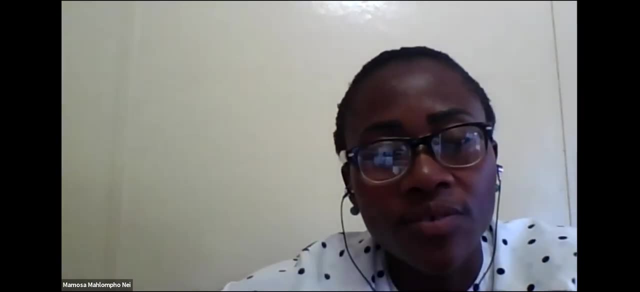 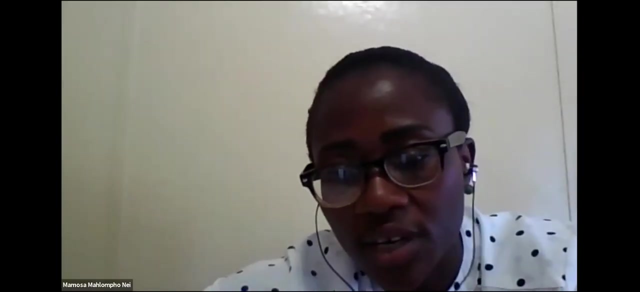 there is a view up there. you click on it. it will show speaker and gallery and then you click on gallery. it will display all the videos of: on my, on my right. it's on your right screen, on the screen up up there at the corner. let me, let me make. 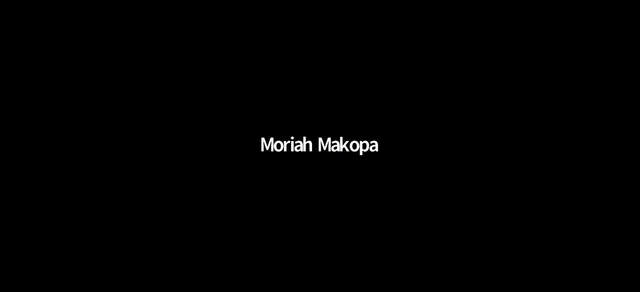 let me make you. course, I, I can see it from this end, but you can make it okay, so please go ahead, Maria. okay, have you found it? yes, I can see view then. then I click on gallery. you go to gallery. yes, I can see everyone now. yes, so it will display every one on the screen, everyone on the screen. 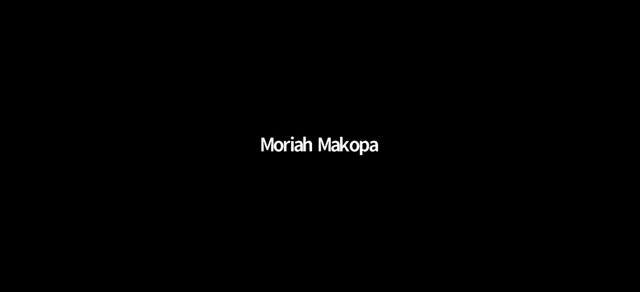 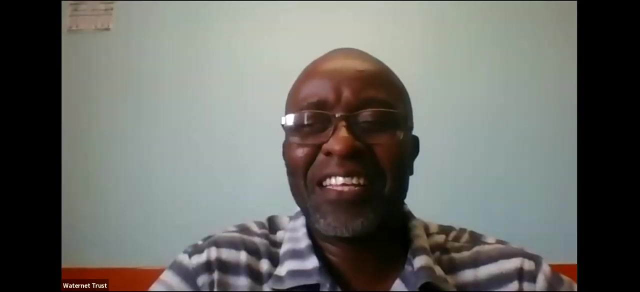 okay, so Maria, can, can you take? can you take the the screenshots please? so it's print screen, it's a screenshot. yeah, screenshots. okay, tell us when you are done. oh, my, my my video is not on, sorry, yes, okay, okay, so people can can see who was talking to them.